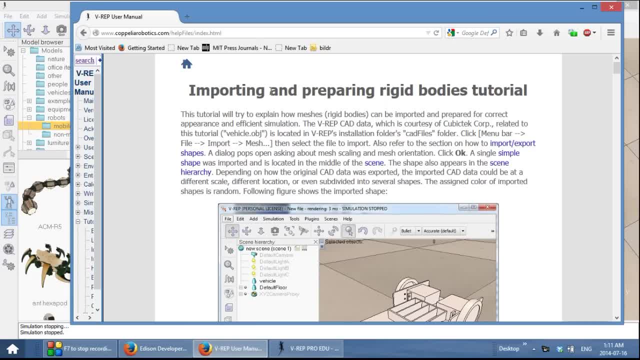 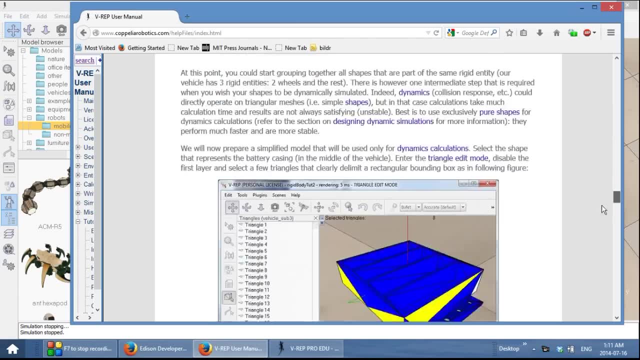 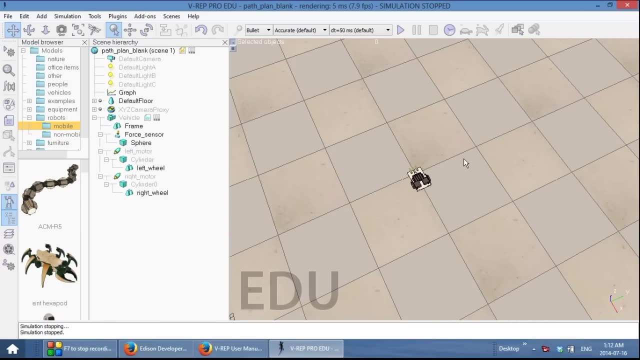 This file picks up where the importing and preparing rigid bodies tutorial leaves off. I have uploaded the file to make things easier on you. if you just want to know about the path planning functionality, The first thing we're going to do is we have to add a couple of obstacles into the field. 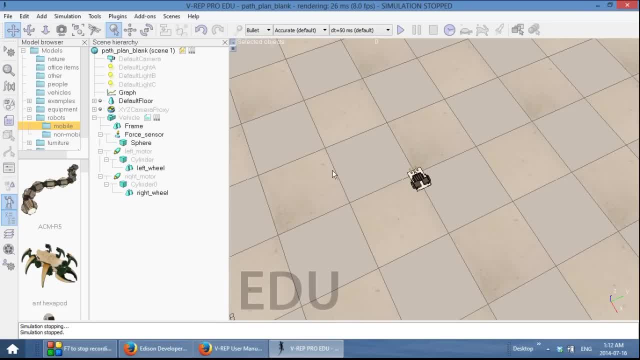 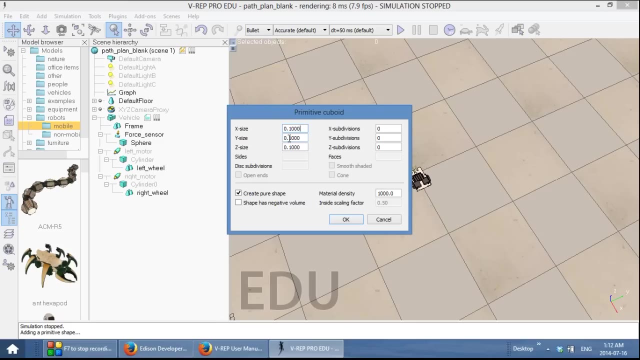 We also have to set the properties of these obstacles so that they're being considered by the path planning module. Right click anywhere in the scene, select, add primitive shape and then cuboid, And then set the size appropriately: maybe 0.8,, 0.1, and 0.1.. 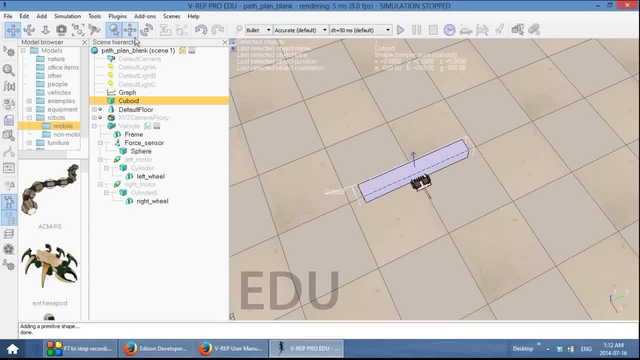 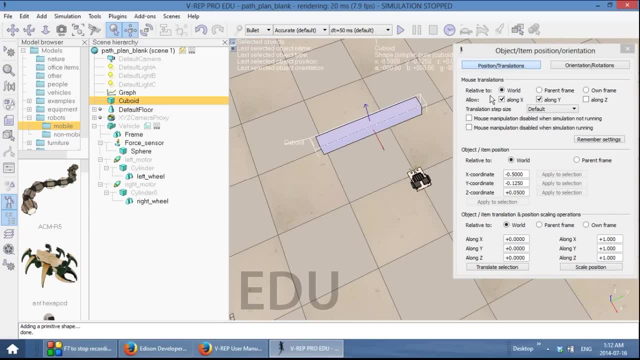 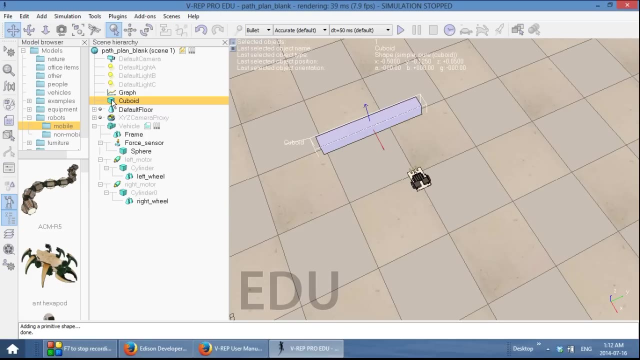 And then you get an object just like that. Select the object item shift and then drag it around. And currently the mouse translations are along the X and the Y axis. Double click on this cuboid icon and set some properties Under common: select collidable, detectable and measurable. 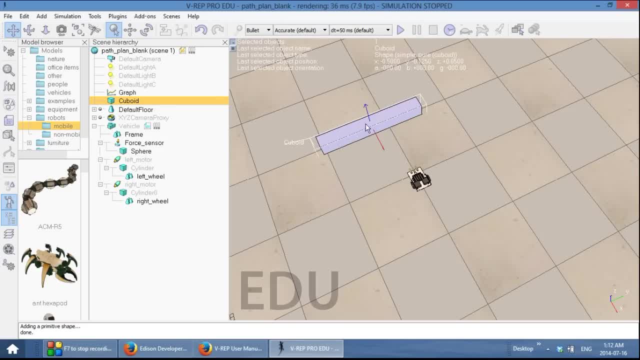 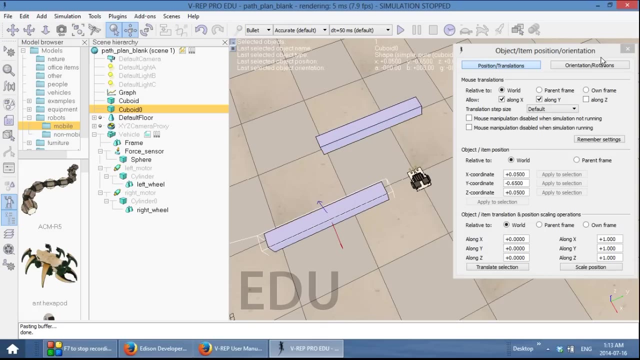 Now, since we don't want to have to go through the process over and over again, one thing we can do: we can select the cuboid and then just press control C And then control V, So essentially we copy and paste the same object with the same properties. 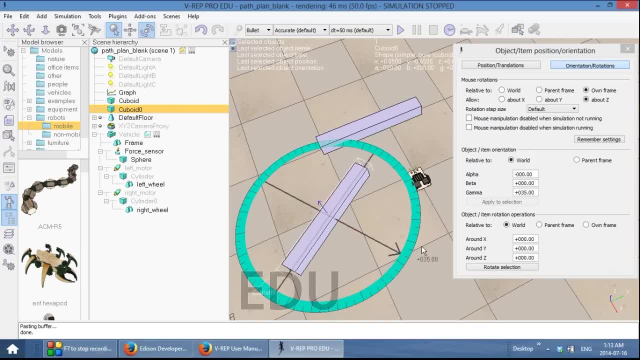 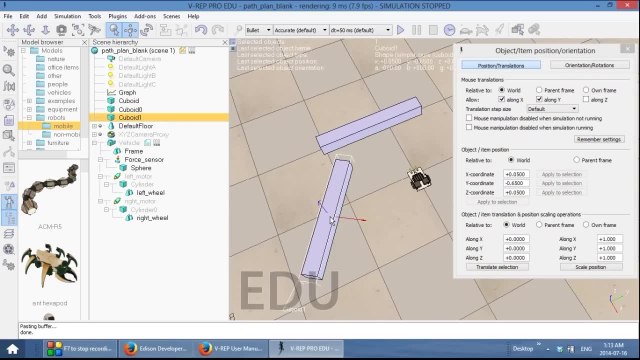 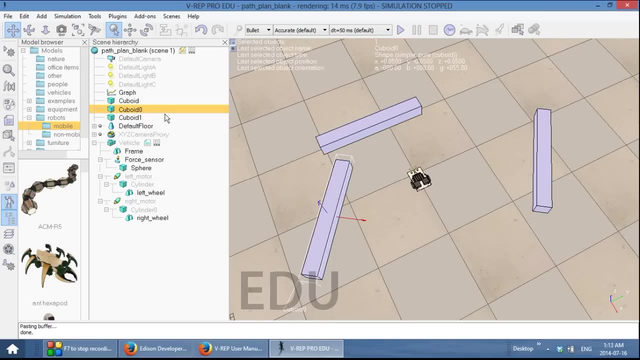 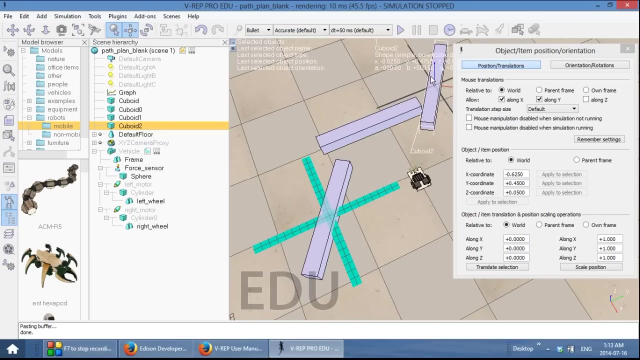 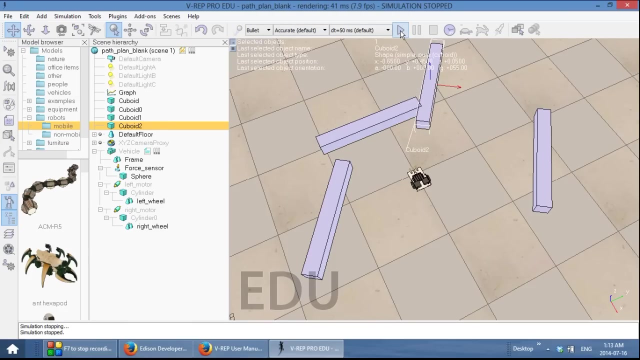 And then we can easily just rotate things around and make a couple of obstacles And make something that is nice enough yet somewhat complicated, So that the path planning module has to work for it. Also, try to avoid any kind of overlap. If you do have overlap, when you run the scene they just they jump apart. 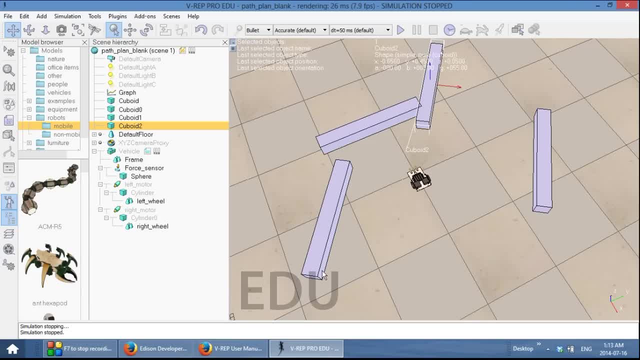 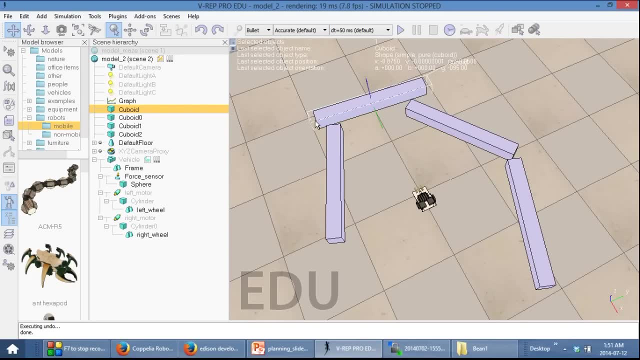 And there you have it. Here is your first couple of obstacles. Now that you have a couple of obstacles in the field, we have to define something that's called a collection. First, we have to make sure that all of these obstacle objects are selected. 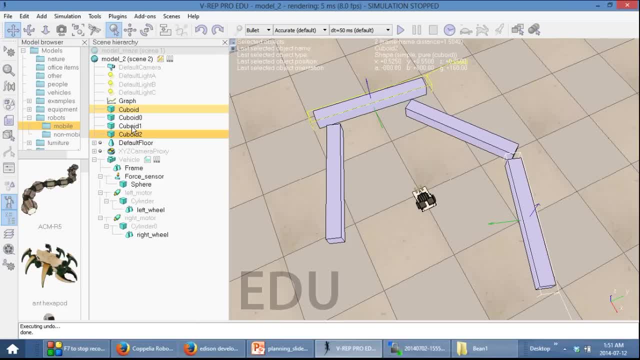 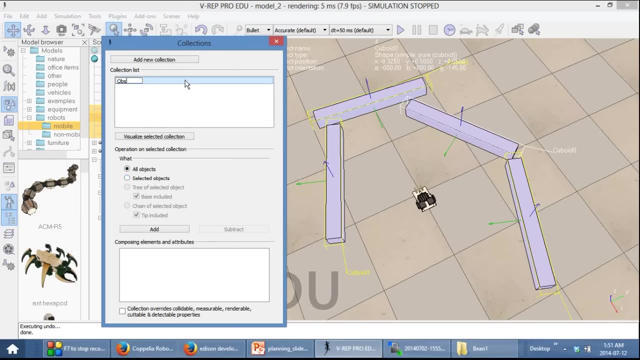 Hold down control and select all of the and click on each of the names of these cuboids. Over here you'll find this button that's called collections: Select, add new collection And then rename it into obstacles And then here under operational selection. 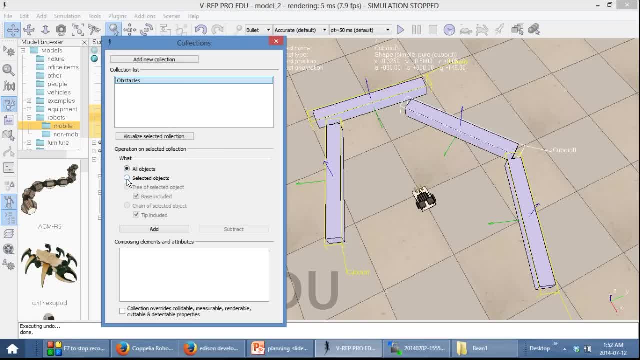 Under operational selected collection, click the selected objects and press add. Now you've added all of these objects into an obstacle collection. This will simplify calculations down the road, And if you want to add any additional obstacles, all you have to do is add them into the collection. 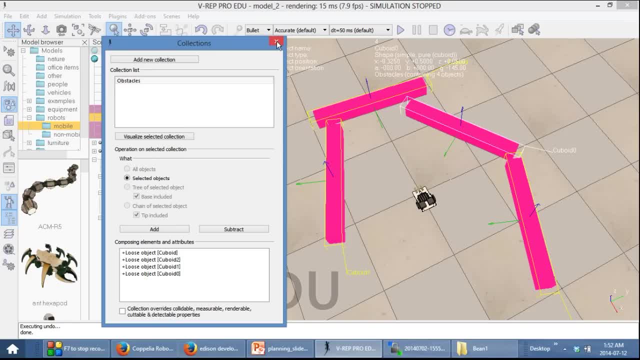 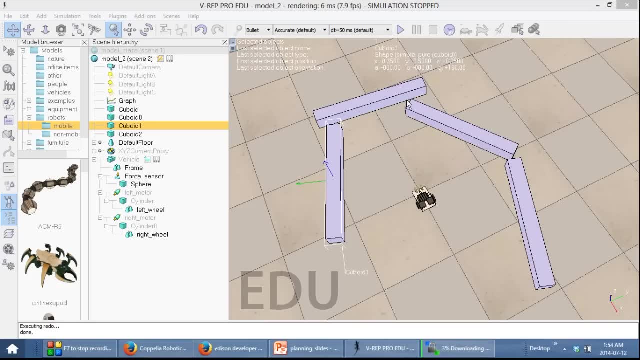 And then the path planning module will later automatically consider them in the path planning calculations. Now that you have a collection of all the obstacles, we can begin with the path planning setup. Whenever you do path planning in VREP, you need three things. 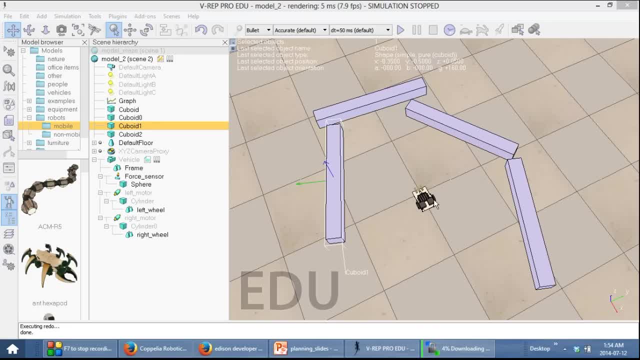 You need one, a starting dummy. Two, you need a target dummy somewhere else. And three, you need a path object. So let's add all of these three items into the environment: Right click anywhere, select add and then dummy. 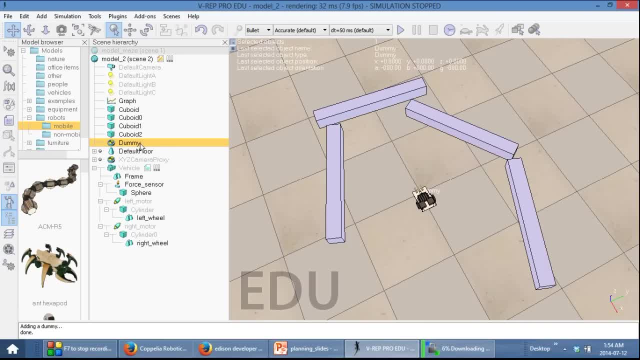 A dummy does not serve any purpose other than well, it's used for calculations. You can rename this as start And we're going to place it in the same position as our vehicle. So, with start selected, Hold down control and select vehicle. 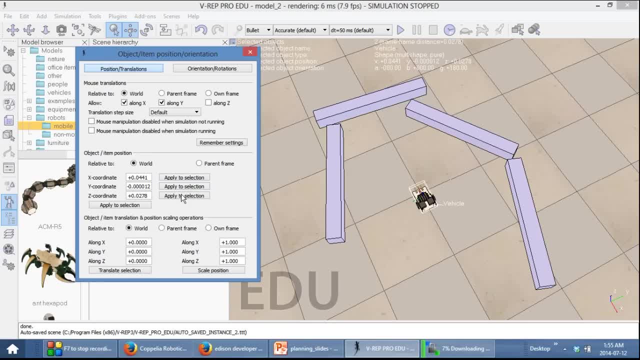 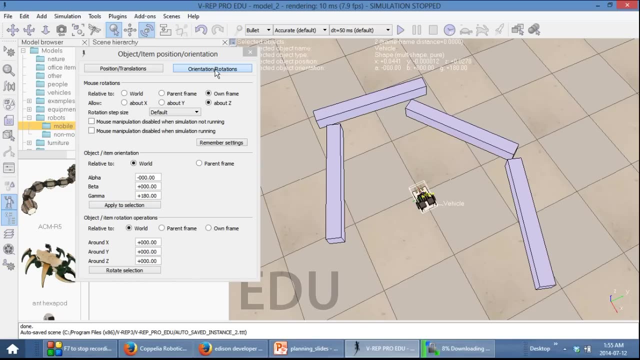 And under position select apply to selection. This will move the dummy into the exact position of the vehicle. In addition, we also want to change the orientation and rotation, And here we select the orientation tab and then click apply to selection. So now the starting dummy has the exact same orientation as our vehicle. 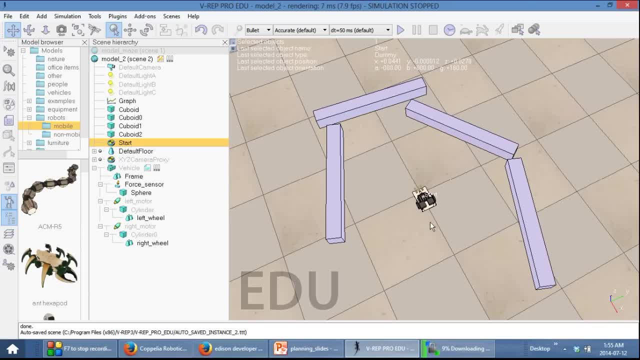 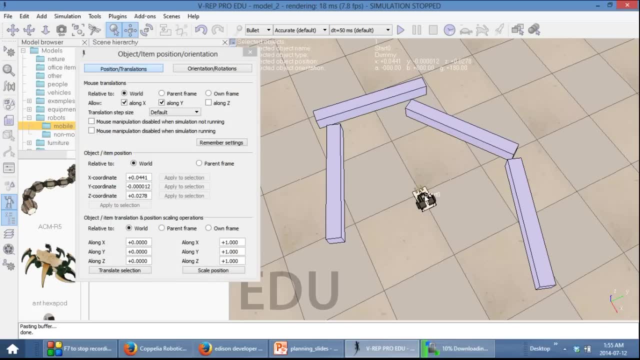 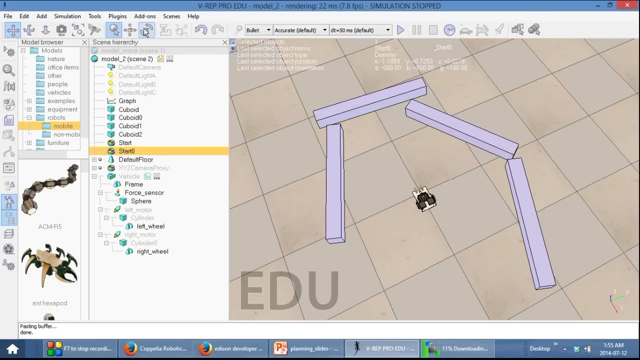 So we can then control C, copy this object and then make a copy in the environment. This will become our target dummy object, So we can drag it around and move it somewhere outside of the obstacles. And one thing we can do, we can also rotate it around a little bit. 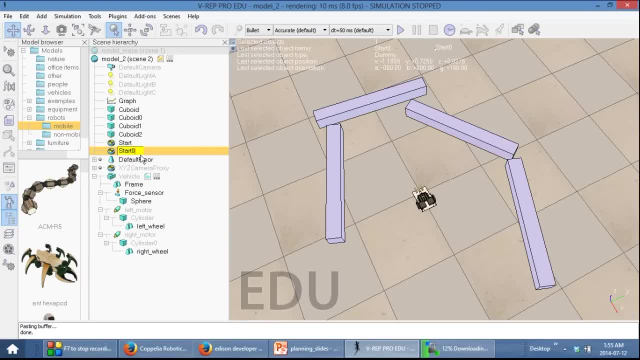 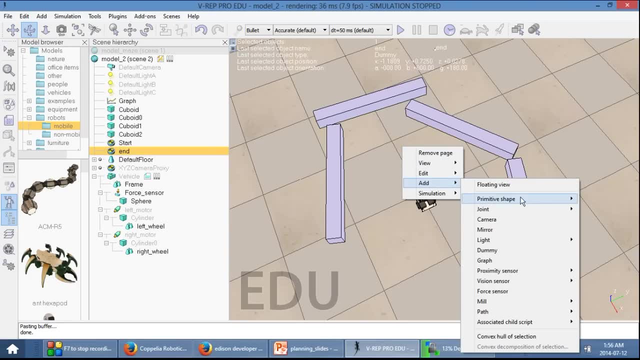 And then let's rename it into end. So then we also have to add a path. Right click and then select add And then path. I'm pretty sure it does not matter whether it's segment or circle type, Because when you run the path planning function it will just overwrite whatever waypoints you have there anyway. 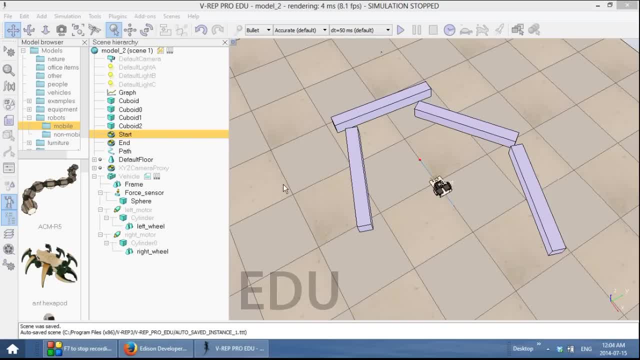 Now that we have all of the obstacles And we have a start configuration, A goal position, which is represented by this end dummy And the path where the path planning module will store its path that it calculates, We can then begin and select this calculation module properties button on the sidebar. 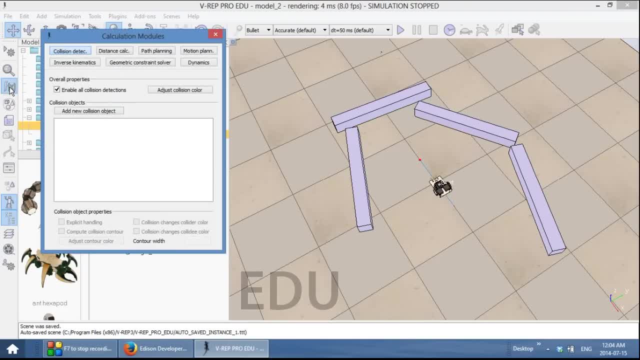 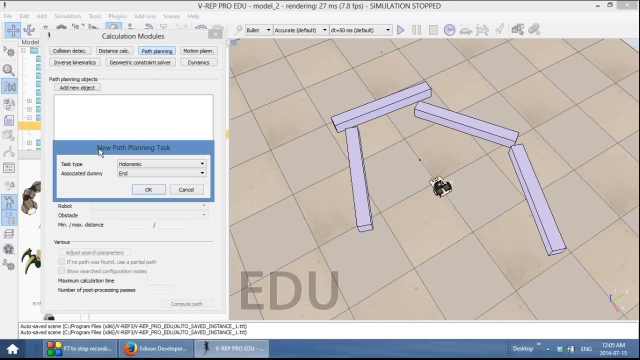 To access some of VREP's advanced functionality. Here you have the collision detection module, the distance calculations, inverse kinematics, motion planning And the path planning module That we'll be using. Select add new object to create a new path planning object. 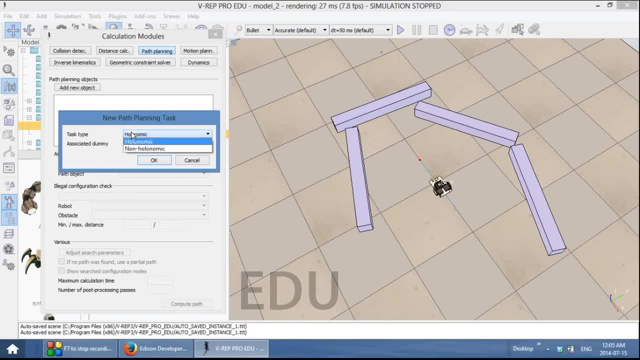 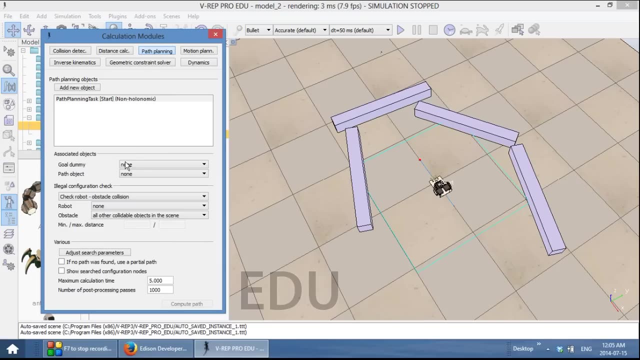 We're using a differential drive robot, Which is a non-holonomic system. As far as the associated dummy goes, Select start, because that's the dummy that we want to traverse along the path. Now select okay. So another thing we have to add is we have to select the target. 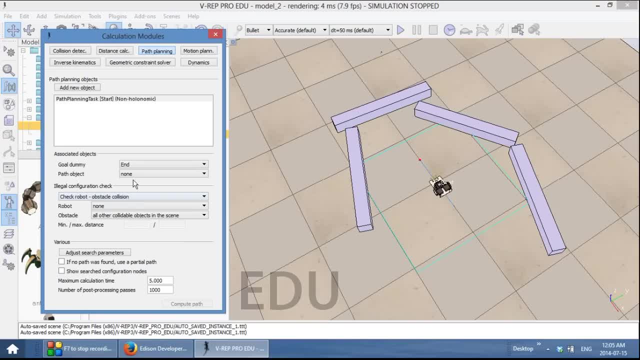 Which we will select to be the end dummy. The path object is the path where it wants to store the path. We select path For now. let's not do anything about the illegal configuration check. Let's look at the search parameters. You might have noticed that there is a light blue box over here. 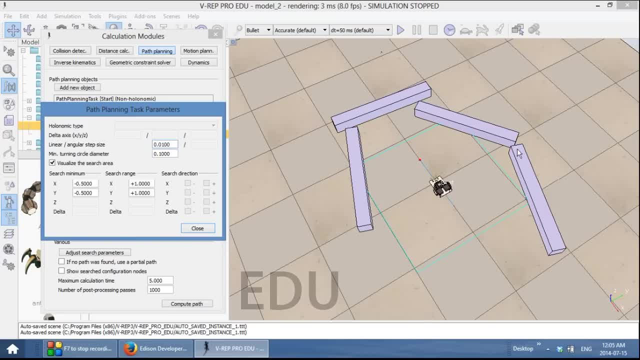 This represents the area that will be searched for the path. Now you might also notice that our target position is outside of this search parameters. So one thing we have to do is we have to increase the size of it. Now, the way that VREP path planning does the search parameters: 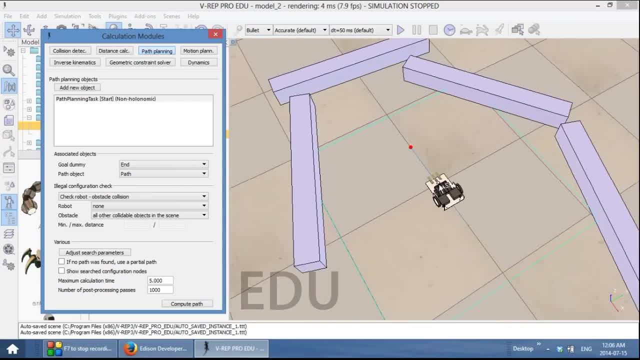 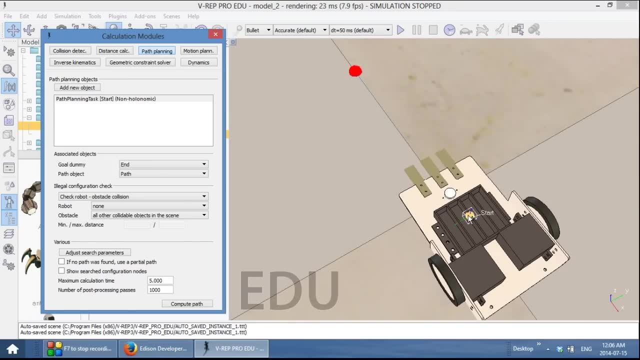 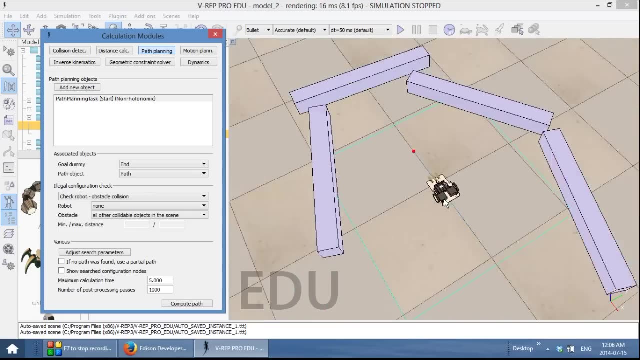 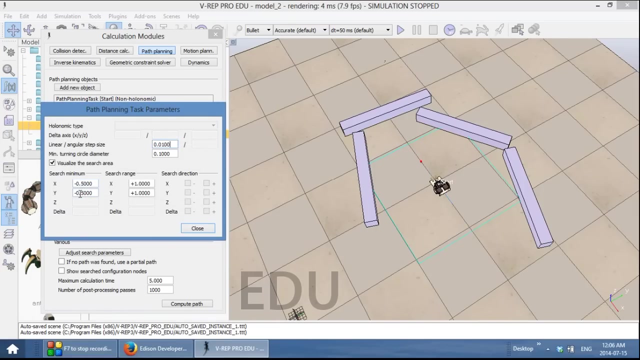 Let me zoom in onto the start dummy. The start dummy shows its y-axis To be to the left And its x-axis to be towards the top of the screen. So over here it selects a point at minus 0.5 and minus 0.5 over here. 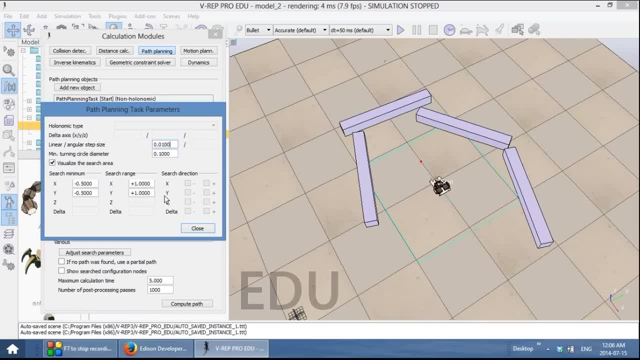 And then it looks for about 1 meter by 1 meter, which is indicated by here. So for now, let's set it to minus 2.. And I found that this box does not update until you select close, And we want the search range to be 4.. 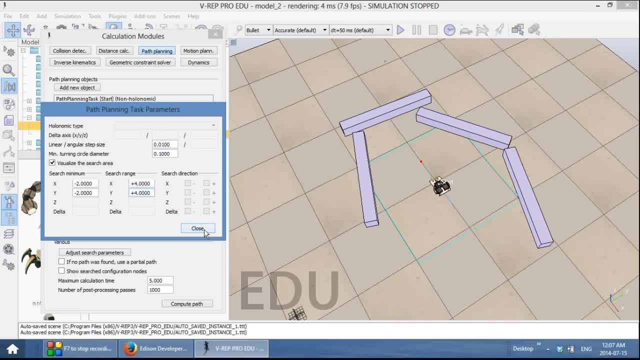 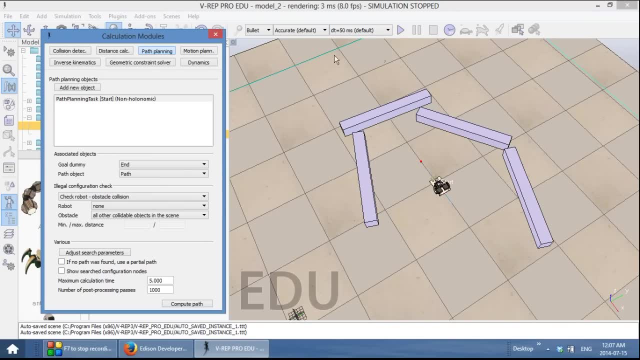 So now we have a much larger box and you can see that it includes everything, Which includes also the target configuration. So what happens if you click compute? again, What happens once we click compute path? If we click compute path, it just connects the start dummy and the end dummy. 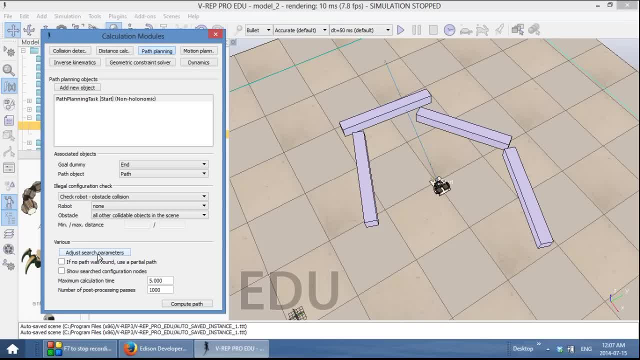 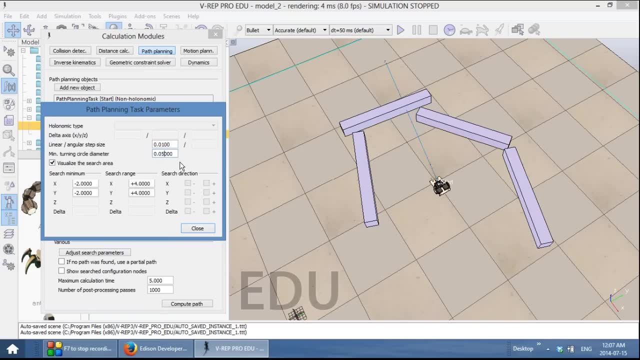 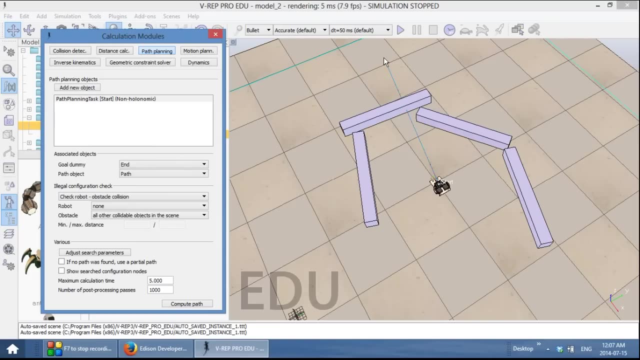 One thing that we forgot to mention and to adjust is here, under the adjust search parameters, is the minimum turning circle diameter, Which I'll change to 0.5.. So for now, you will see that this path currently goes through the obstacles. So one thing we have to do under illegal configuration check. 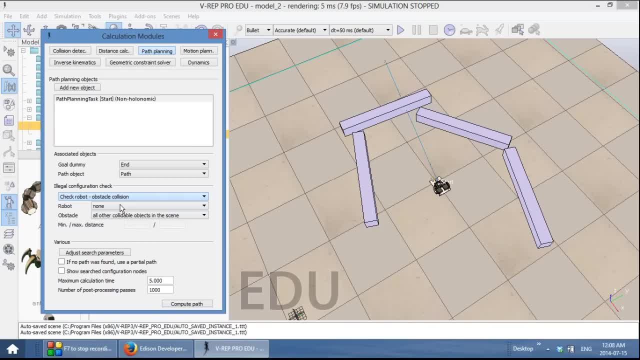 Let's say, check robot obstacle collision, And then under robot we select the frame And under obstacle we select collection, And now we click compute path And you'll find that it still shows up as the path goes still through the obstacle. I've done this on purpose to illustrate a couple of things. 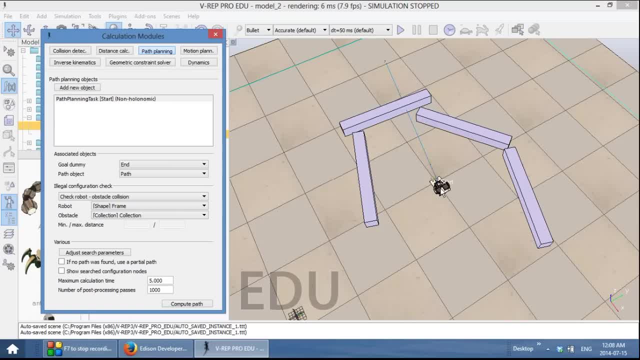 What VREP does? it takes the start dummy and then traverses it along its path And at every step along the way it checks the obstacle: robot collision. So, for example, now the start dummy moves to here And it checks whether the robot has collided with the obstacle. 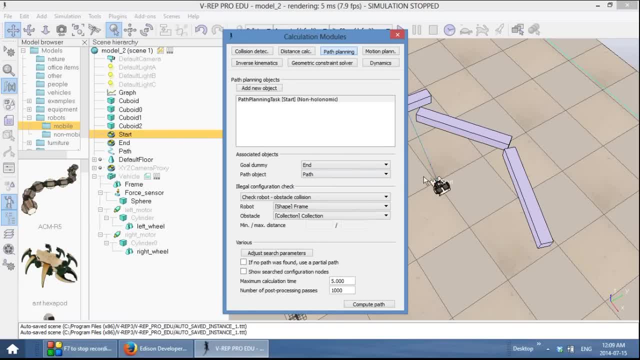 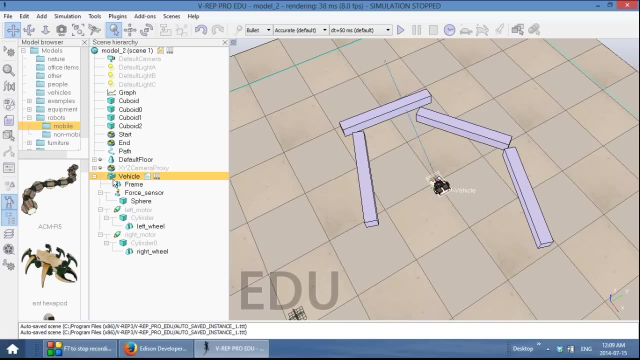 But you will see that for now The vehicle is not actually attached to the start dummy. Thus when the start dummy moves, the vehicle stays behind. So to fix that we have to make the vehicle the child of the start. You can do that by grabbing the vehicle and dragging it onto the start dummy. 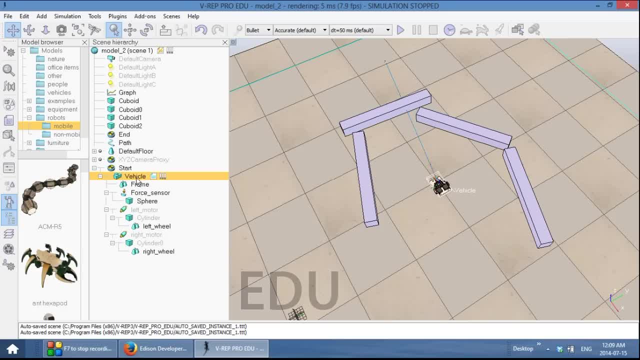 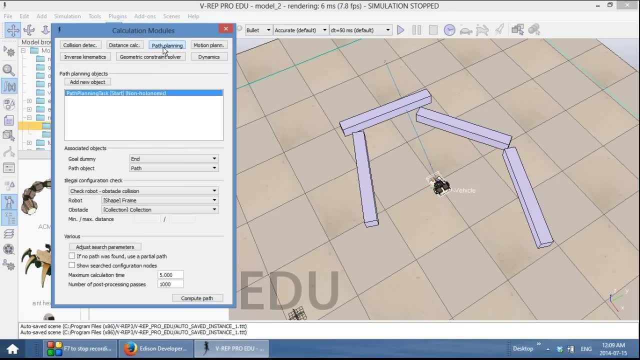 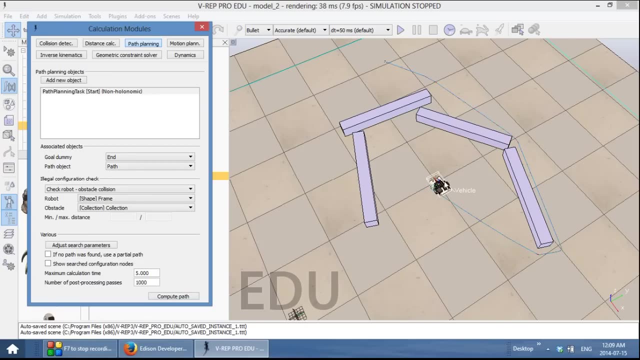 So now we made the vehicle the child of the start dummy. So then, when you click path planning Now you can recompute the path, And now you'll see that it actually found a path that goes from the start configuration all the way to our goal. 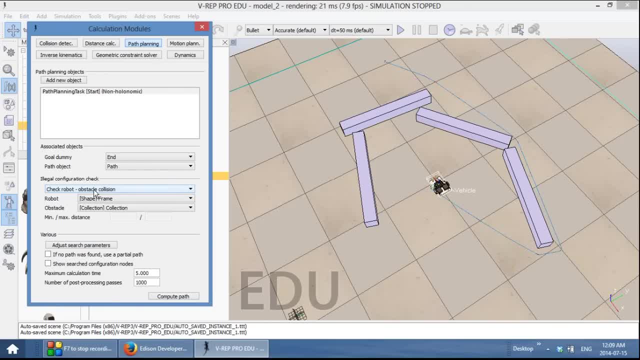 You can play around with some of these properties. For example, this check robot, obstacle collision- just checks whether it has collided or not, So it tries to get it as close as possible to the obstacle. You can also indicate an obstacle- minimum distance, So, for example, if you want the robot to take wide turns. 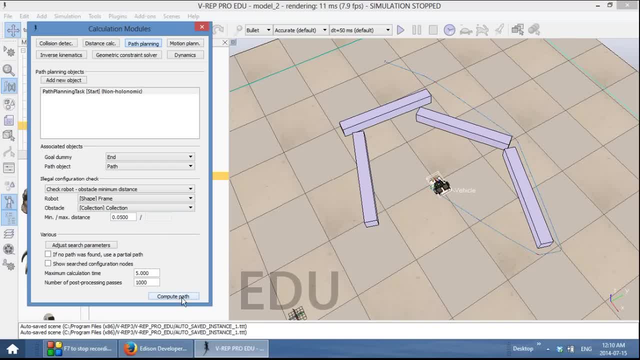 You can try and compute that, Maybe make it a little bit larger, And now it's a little bit too much currently, So it didn't find anything, But let's just set it to 0.1.. And now it will try to avoid the obstacle by approximately 0.1 meters. 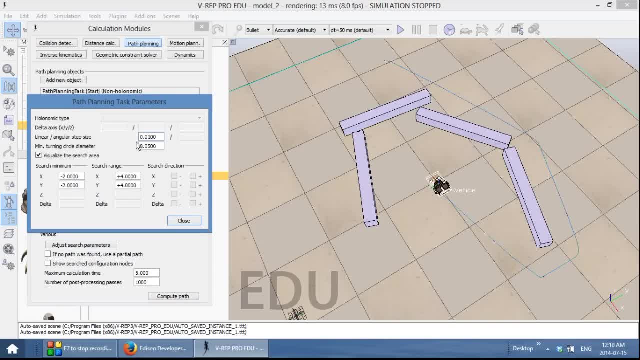 Another thing that we can also change is the minimum turning circle diameter. That's, how much of a turning circle does your robot need? Now, for a differential drive robot, this does not really really matter, But if you have something like a car steering, that becomes a parameter that you might want to look into. 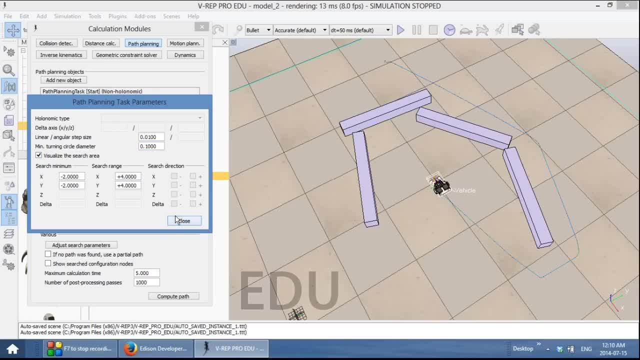 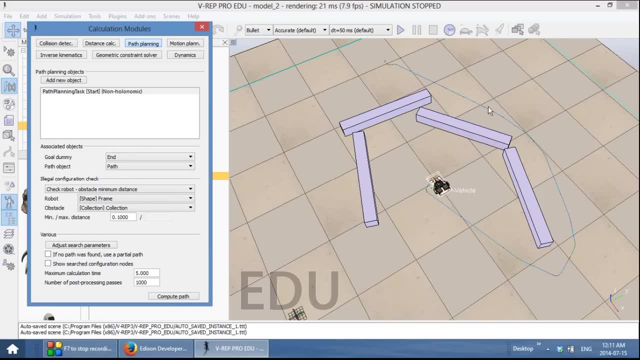 So what happens if you set it to 0.1.. You can compute the path, And you'll find that some of these corners are now a lot less sharp. So there you have it. So all you've done now is you've computed the path that goes from the target to the goal configuration. 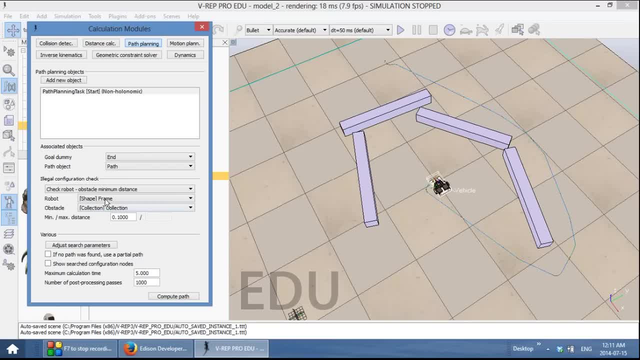 While avoiding all of the obstacles in between. You can also see why it was important to just To define the obstacle collection. I should mention some properties of the path planning. object: Down here you have maximum calculation time, Which is how long in seconds before the processor gives up to try and find the path. 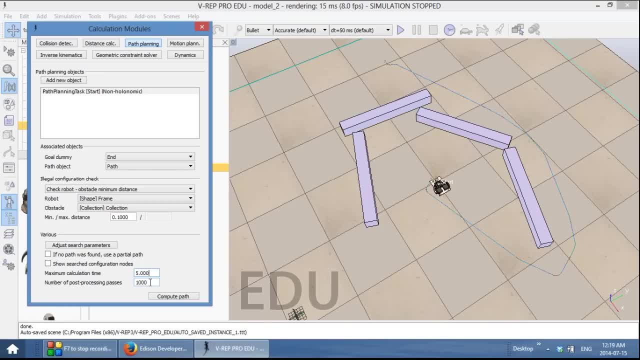 The number of post processing passes Is how many times the path planning module will go over a certain path. To try to simplify it, This option right here, of no path was found, use partial path Will get the robot to the closest possible position to the object. 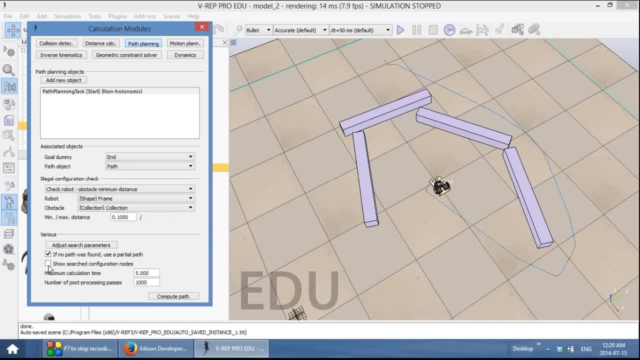 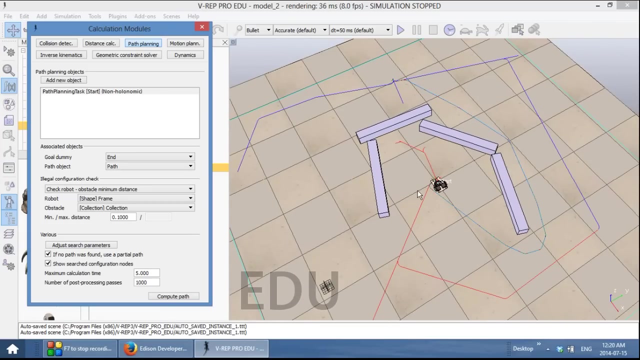 Or to the target. Another very interesting option Is show search configuration nodes. If you select that one and click compute path, You will see all of the options that VREP has considered while trying to find this path, And you can kind of get some insight into how VREP does its path planning. 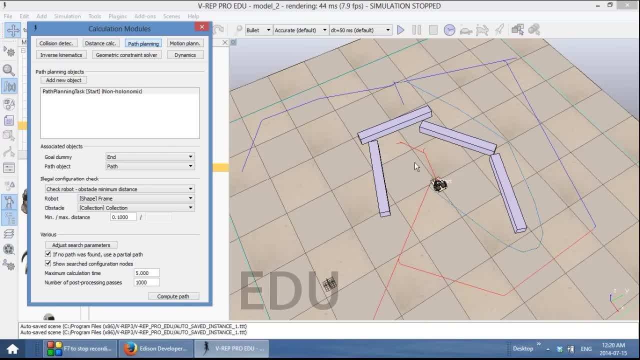 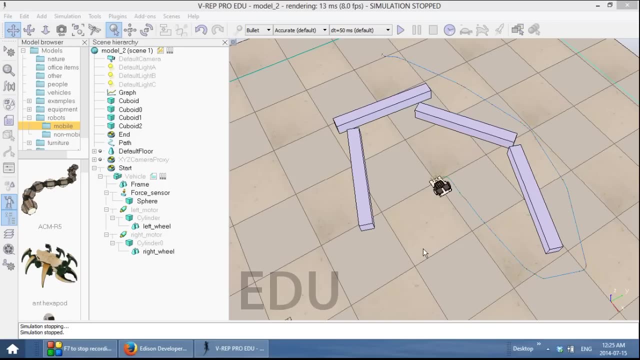 Essentially, it tries all of these different types of paths And then finds whichever one is the shortest path Or the shortest one. Now you have a path that connects your start configuration To your goal, configuration That avoids all of the obstacles And that follows your appropriate turning radius. 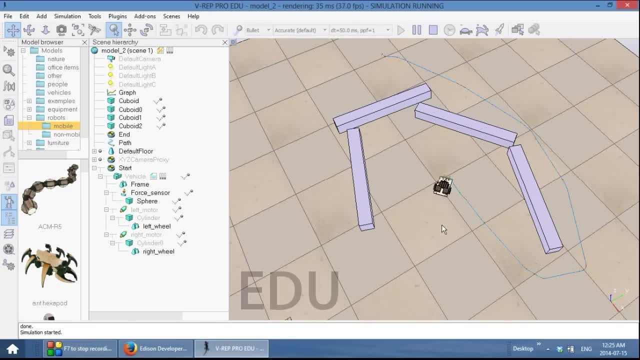 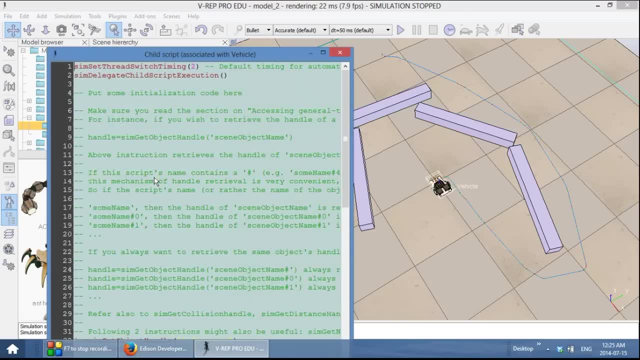 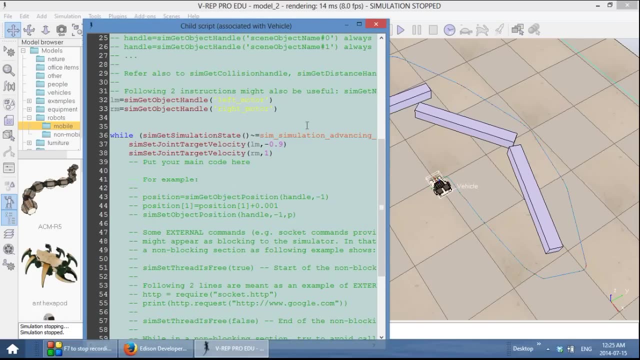 Now, if you were to run this simulation, You will find that the robot just kind of turns in circles, Which is exactly what we programmed it to do. If you check the code for the vehicle- All that it says Here- it says the joint target velocity to 0.9 and 1.. 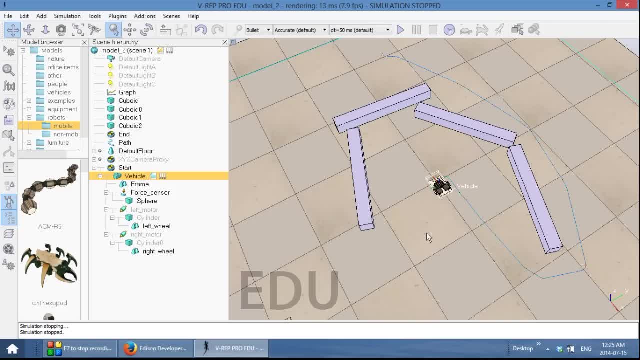 So now there's many options of making the robot follow the path, And in this video I will present you two of them. The first one is to select the vehicle as a static object, And then it will get dragged along the path By its parent dummy object. 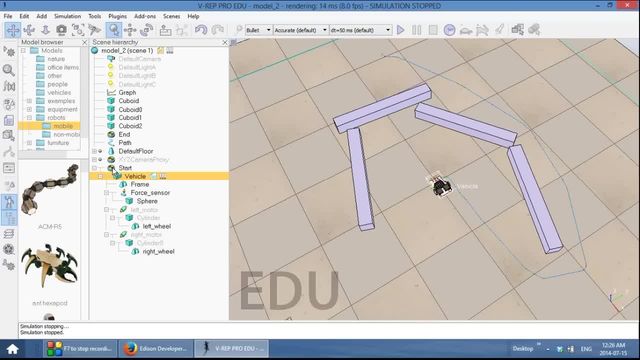 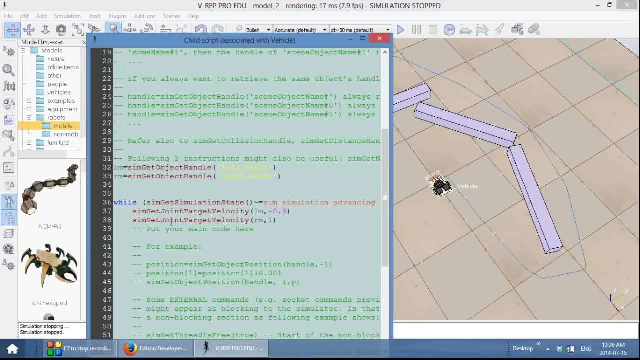 This is not a good way of doing it, But it might work in some instances. If you're just trying to make a quick simulation- The second option- I will actually show you How to set the appropriate wheel velocities In order to make the robot approximately follow this path. 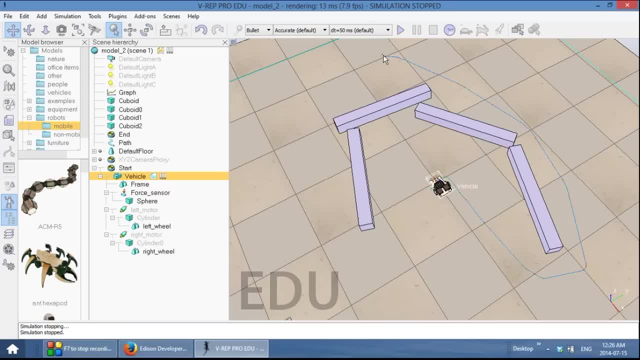 And that will be the second option That I will show you at the end of the video. To make the robot follow the exact path As a static object, You first have to indicate the velocity With which the object should travel along the path. 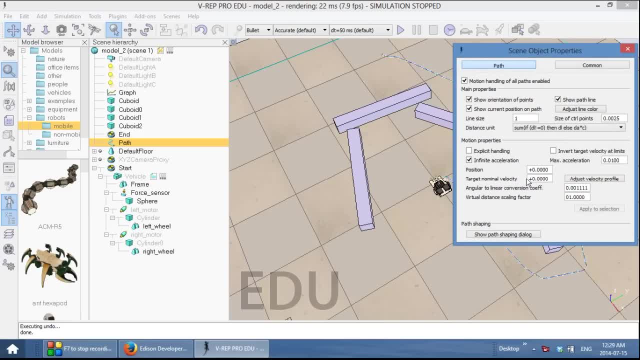 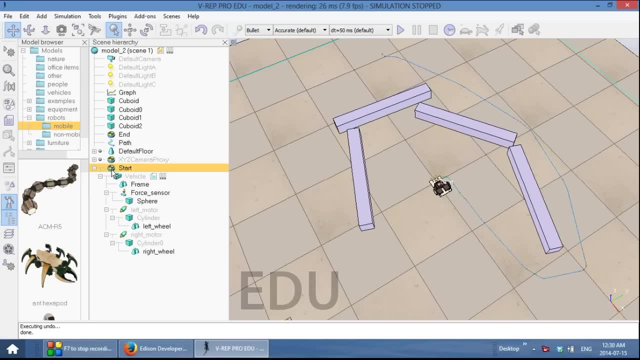 Double click on the path object And, under target nominal velocity, Select 0.1.. Now we have to make this start dummy The child of the path. So select it And then drag it to the path object To make it the child. 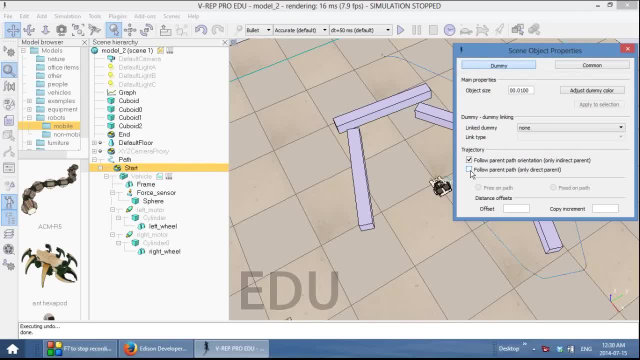 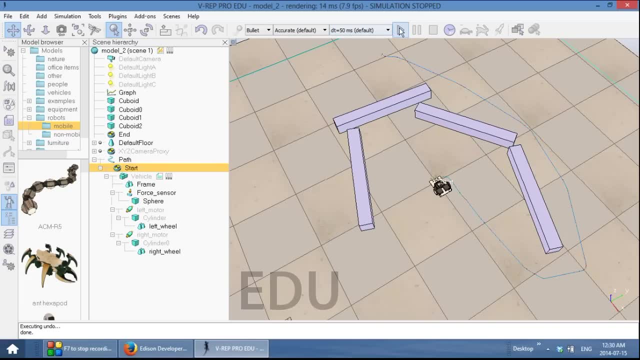 Now double click on start And select follow parent path And also select fixed on path, If it's not already. When you press play, You now can see the start dummy Kind of move along the path And the robot still just turns its wheels. 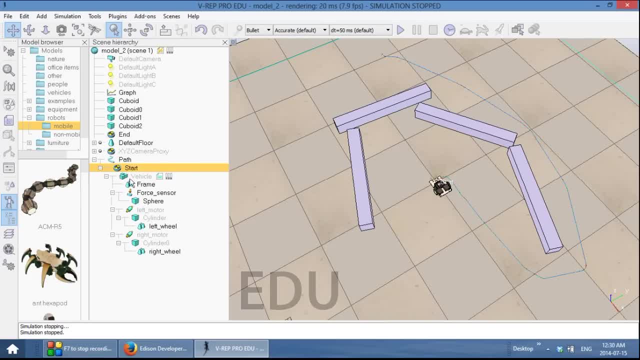 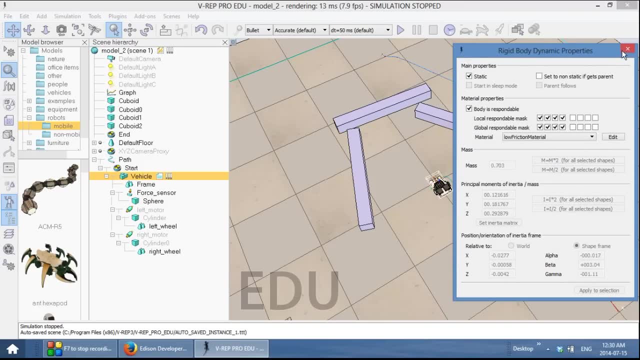 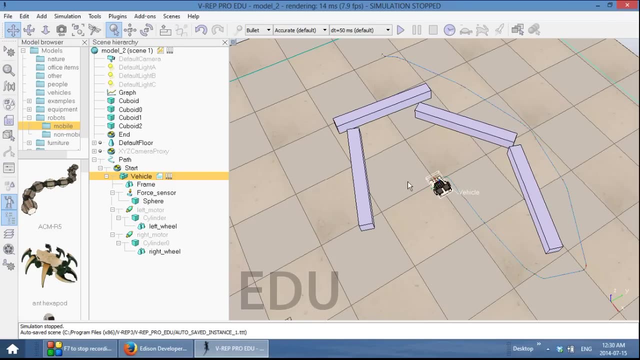 If you want to fix that, Double click on the vehicle And select under show dynamic properties dialog, Select static. This will override anything else that is going on. This will override The fact that its wheels are spinning. So now, when you press play. 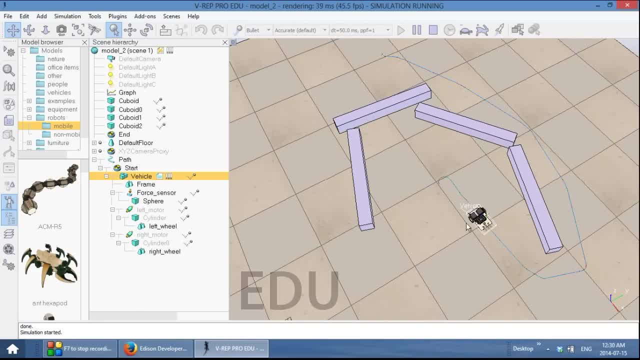 You just see the robot follow The start dummy, Which is its immediate parent, And there you have it. This is the first option On how to make a robot follow a path. Now again, This might not be the best option, Because this essentially forces the vehicle. 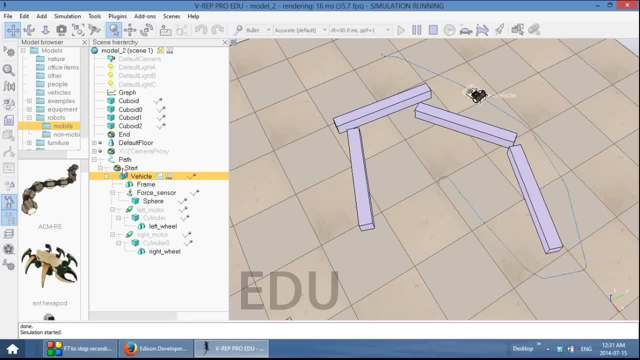 To move along this path. Whether this is a differential drive robot, An airplane Or just a simple cuboid, It will always behave the same. So this might not be the best option. The better option Is to actually design a controller. 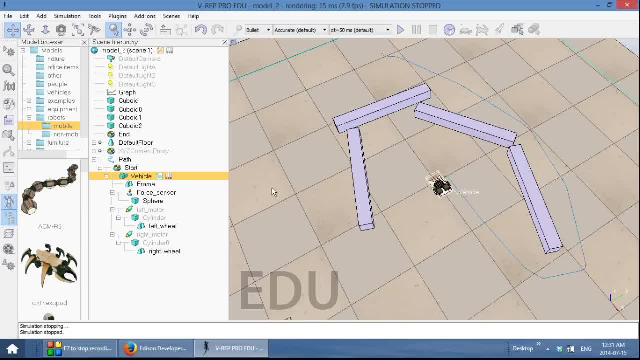 That will send, for example, Wheel velocities To the robot To actually follow the path. And this is the Option That I will explain to you next. To implement a differential drive robot controller, We first have to set the robot Back to static. 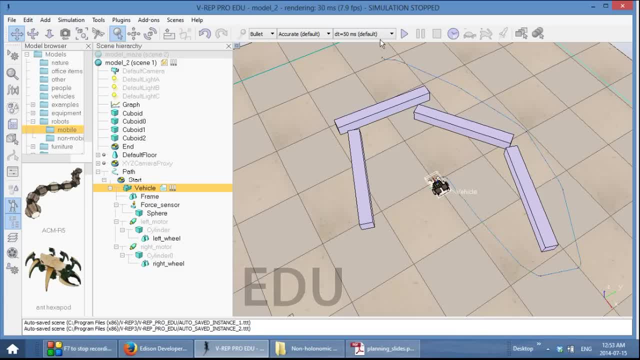 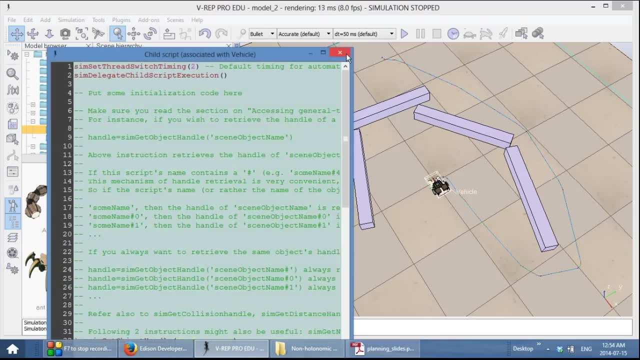 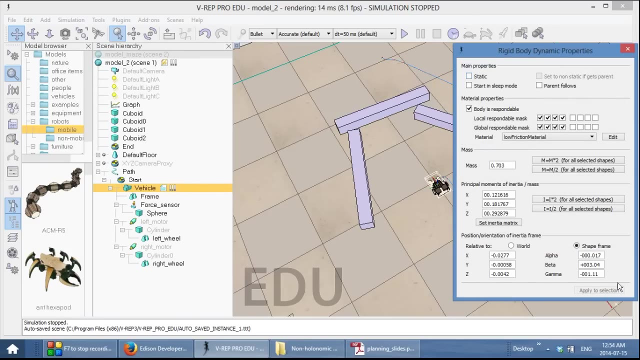 To non static, Because right now It's just being dragged along. So double click on vehicle- Oh sorry, On the vehicle object And then under Show dynamic properties, dialog, Select static. And then we probably Don't want the start node. 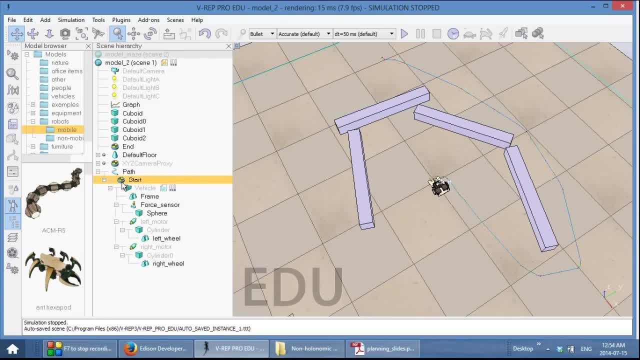 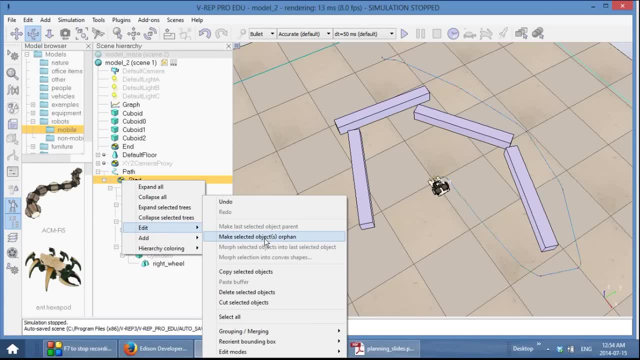 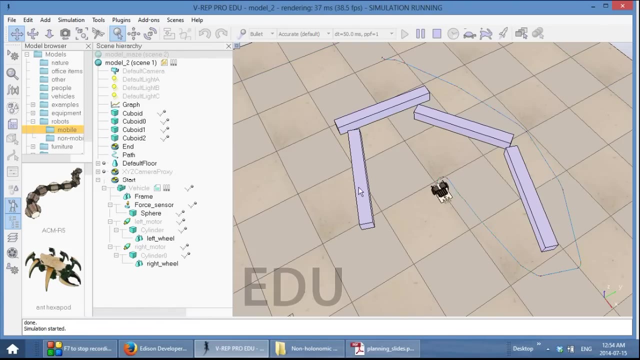 To be the child of the path. So you right click on it, Select And then Edit, And then make selected object orphan. So now The robot continues to turn In a circle, Because that's what we have set: The left and right. 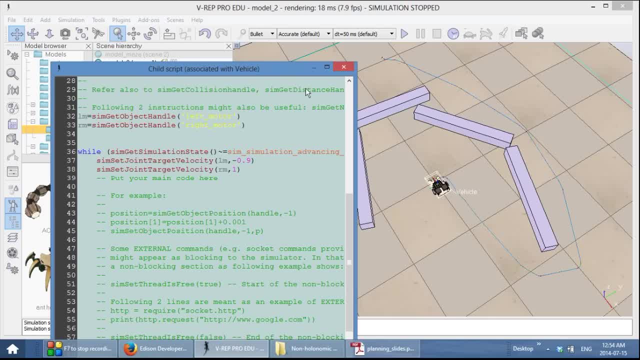 Joint velocity. to Now this joint velocity. I've already set Preset In the file, So now the task becomes: How do we calculate This velocity To make the robot follow Around this path? The design of the controller. 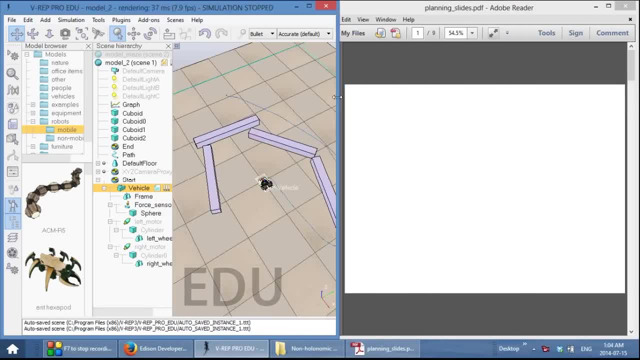 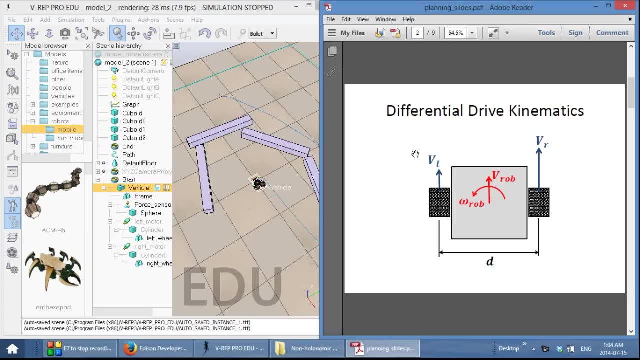 Requires a little bit of explanation. Shown is a diagram Of a differential drive robot And I'm going to explain to you The differential drive robot kinematics. The robot has A forward velocity v And a rotational velocity omega. Now it has 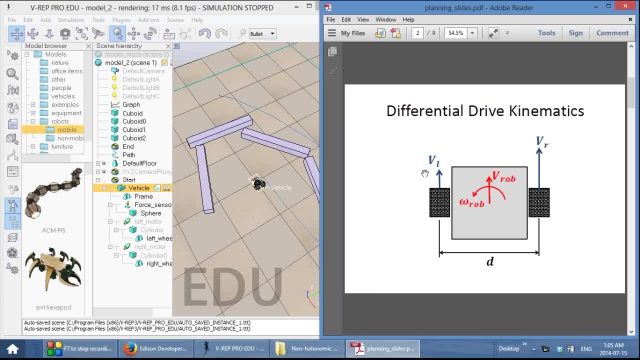 Left and right wheel velocity, Vr and vl, And both wheels are separated by d, Which is the distance in meters. Now the forward velocity Of the robot is just the average Of the left and right wheel velocities. The rotational speed is just the difference. 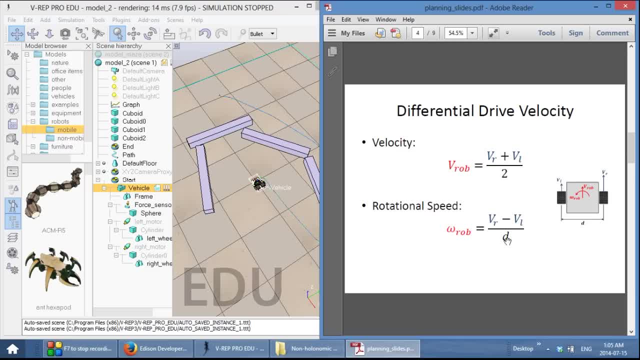 Vr minus vl Over d. Now, ideally we would like to Calculate vr and vl Based on What we want our desired Forward velocity And our rotational speed to be, So thus we can just solve it this way. So those two equations. 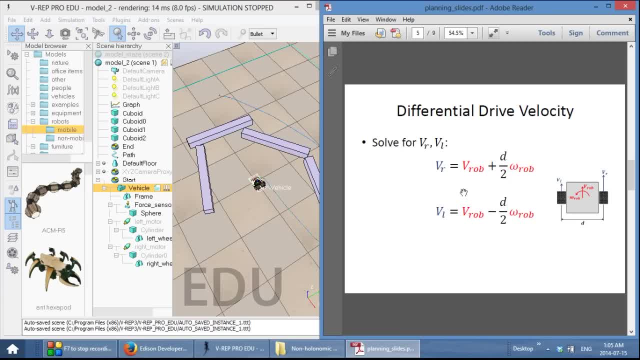 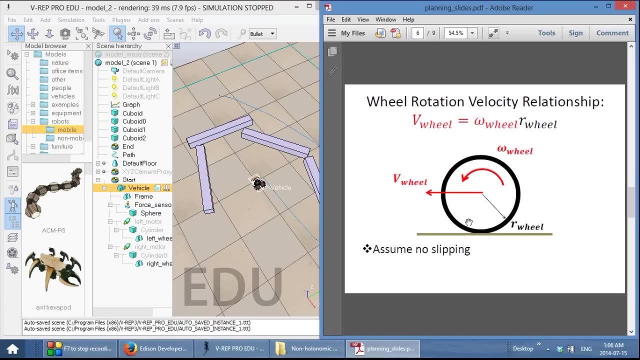 You can solve them out for yourself, But All they do is you plug in your desired Forward velocity And your desired rotational speed, And this equation will give you Your left and right wheel velocities. Now, Since vr Takes in a wheel rotation, 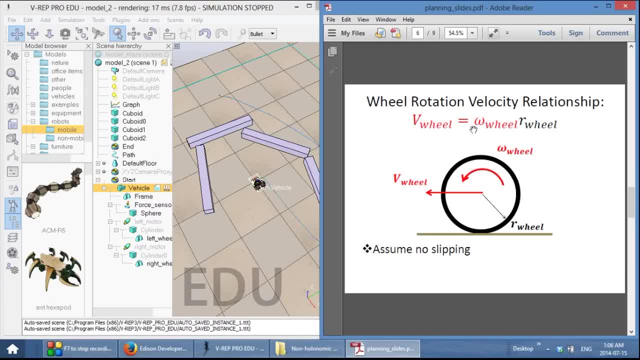 You have to convert those wheel velocities Into a rotation. The wheel rotation velocity Relationship is shown here. The velocity of a wheel center Is just The rotational velocity of the wheel, Times the radius of the wheel. So we can solve. 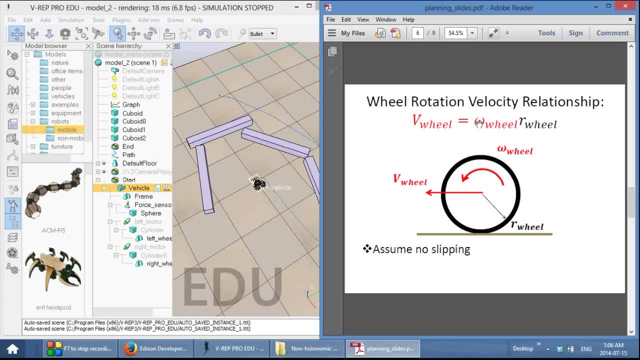 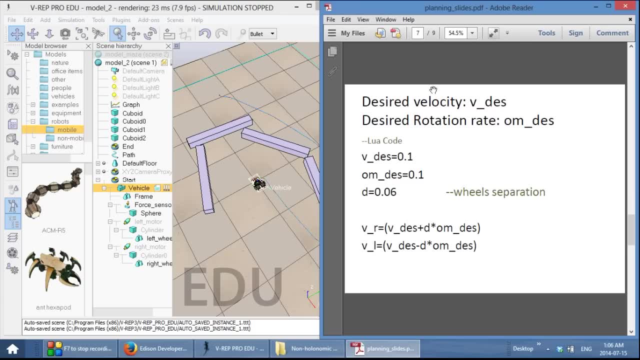 For the desired Wheel rotation By saying v divided by r. So what does that look as Luau code? So first We have a velocity And a rotational speed, And I chose 0.1. For now, just as a sample values. 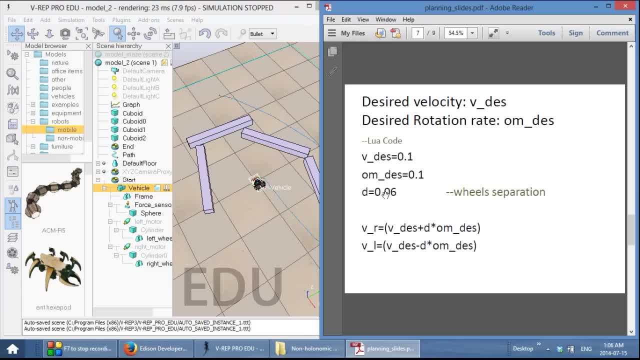 And the wheel separation For this robot Is 0.06 meters, So we can calculate The left and right velocities According to the equation That I previously shown As vdes plus d times omdes And the other one. 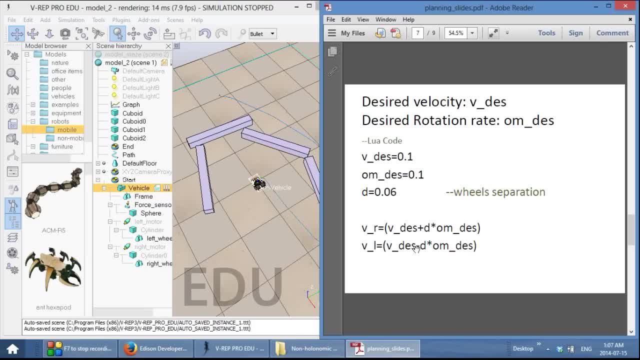 Is just a difference. It's a minus instead of plus. So Once we have vr and vl, We then go on to the next slide. So here we have Rw, which is the wheel radius, So our Right, And this is supposed to be. 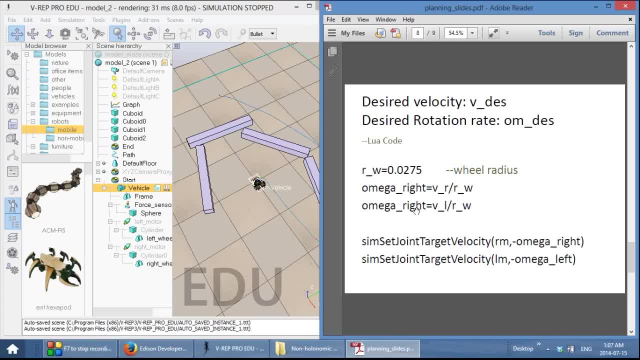 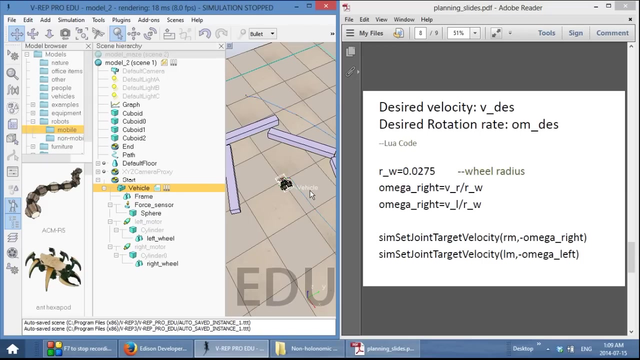 Omega left Velocity is supposed to be Just vr Divided by rw And vl divided by rw, And then you can set The joint target velocity In the code As the follows: So now let's add all of this code. 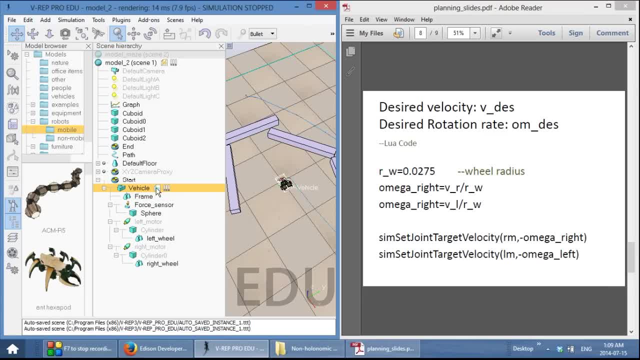 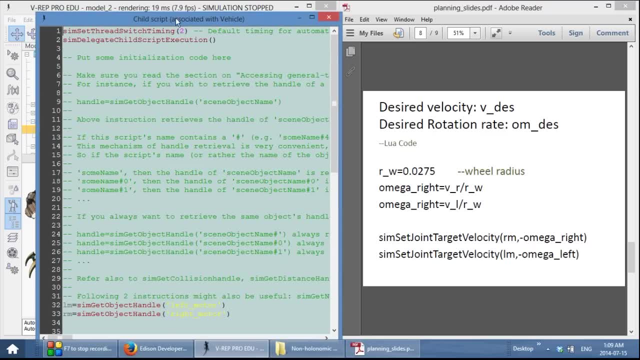 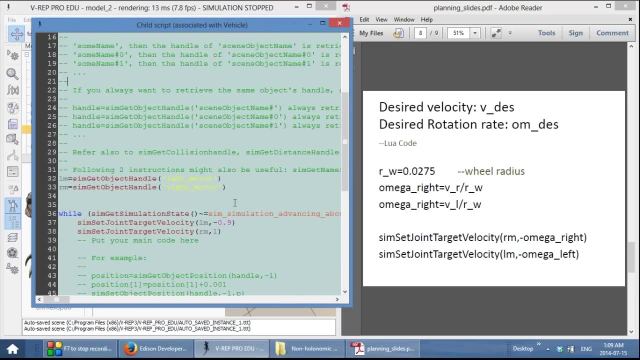 Into our simulation. Now, double click on the Script icon By the vehicle To bring up the child script, Which is associated with the vehicle. This contains All of the programming That you will be doing. Scroll down To the while loop. 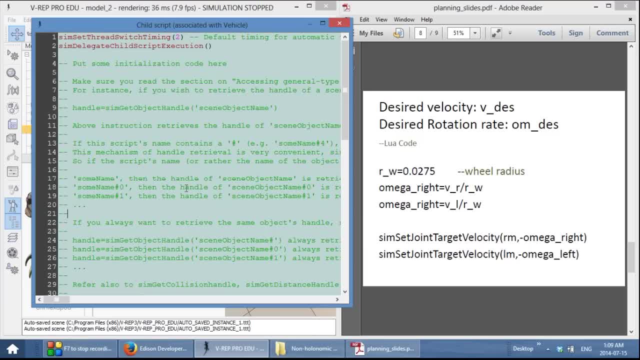 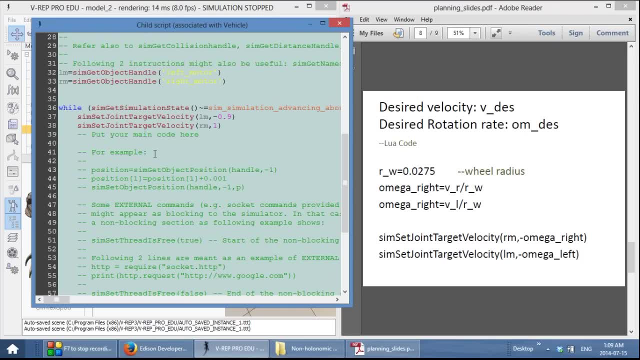 So this child script Is divided into two sections. The first section is some Initialization code, And then there's a while loop Which will run throughout the entire simulation. Currently, all that it does, It sets the right and left wheel velocity. 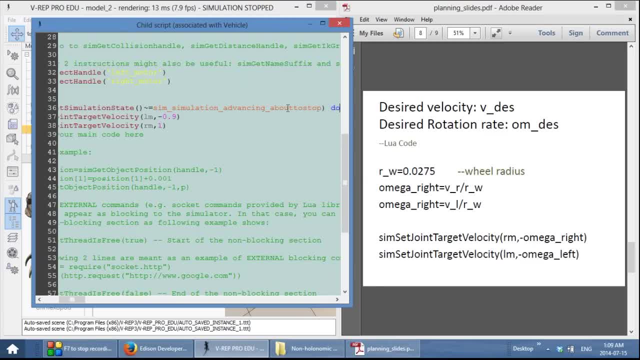 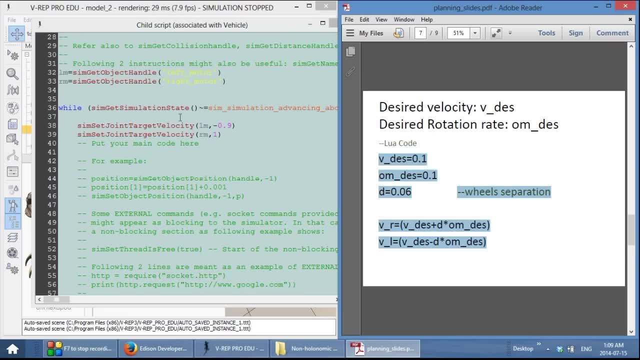 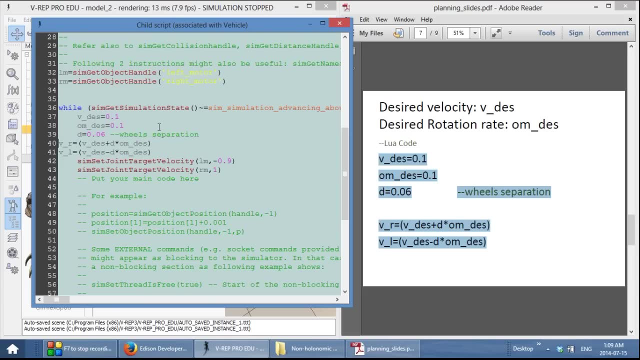 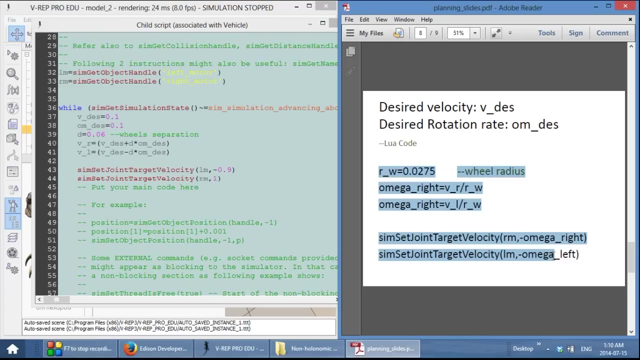 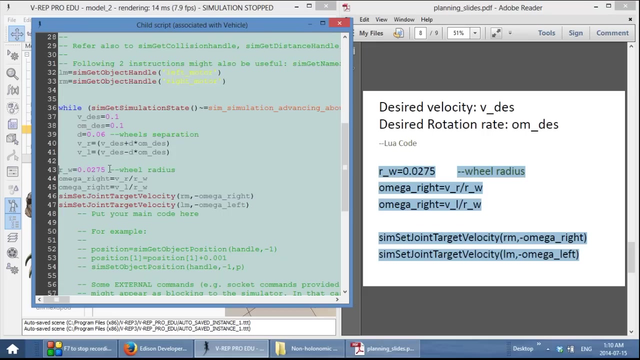 To 0.91.. So Let's add the first half Of this code And then the second half, And this we have to again Change to left Because of the typo previously. Now In the initialization code All we have is: 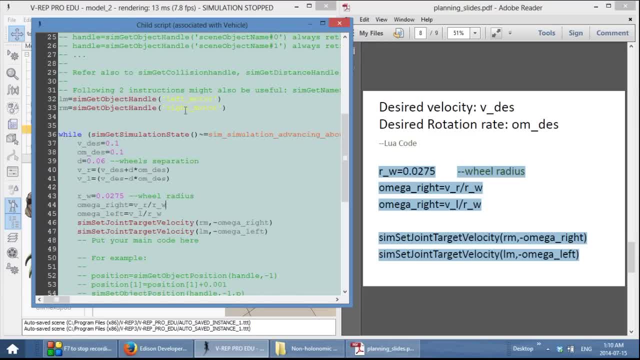 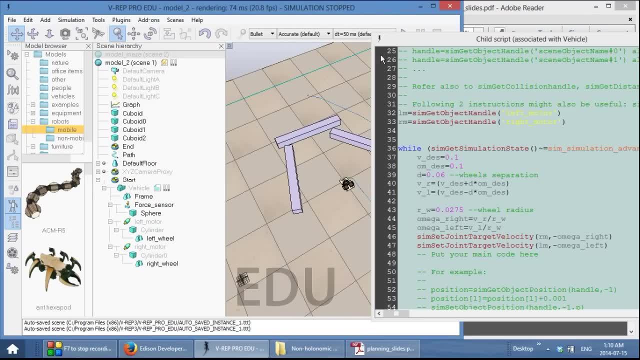 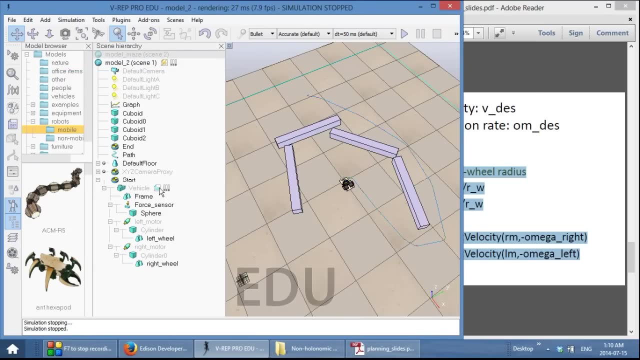 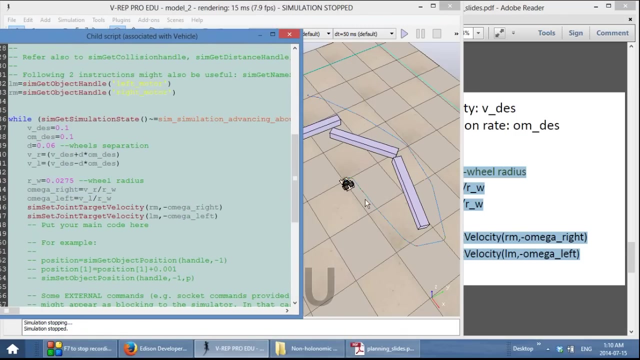 We get a object handle To the left and the right motor. So now let's see What happens when we run this. And now The robot moves forward With 0.1 meters per second And a rotational rate of 0.1.. 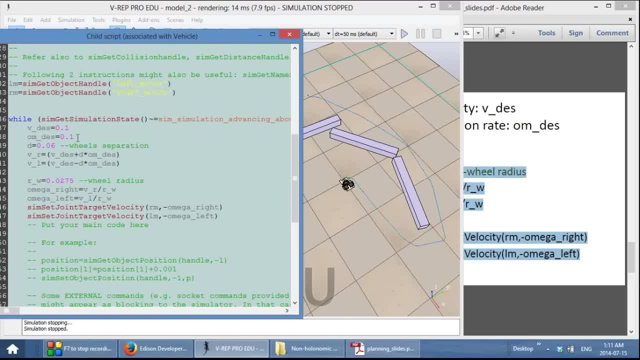 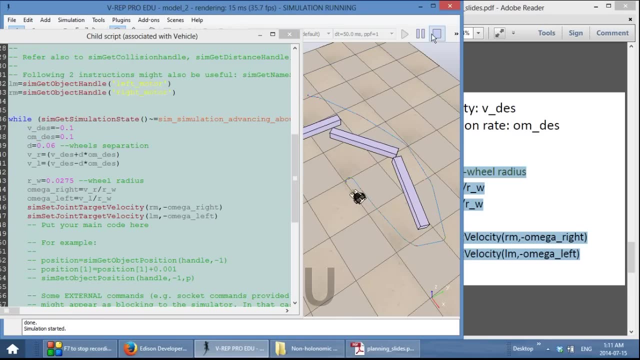 I don't Exactly Remember if it's degrees Or radians per second, But I'll add it in the. I'll make a comment right here. So one thing you can do: For example, you can have it go backwards. So 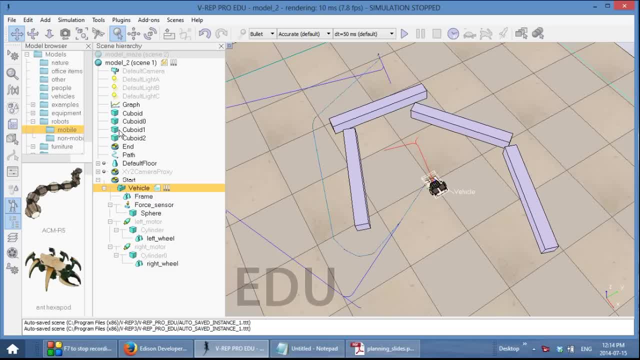 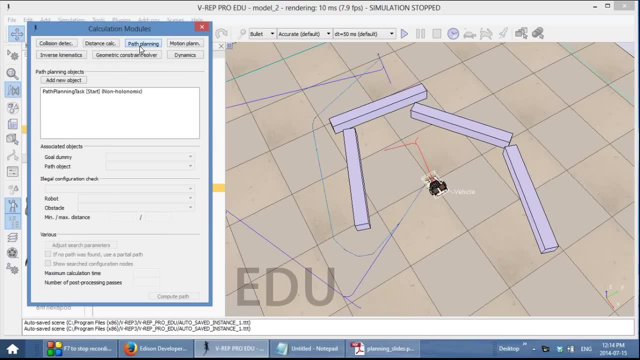 Let's add a path planning dialog From the lua script. Before you can use any of the lua Script functions, You have to first make sure That your path planning actually works. So go into the calculation modules And when you press, compute path. 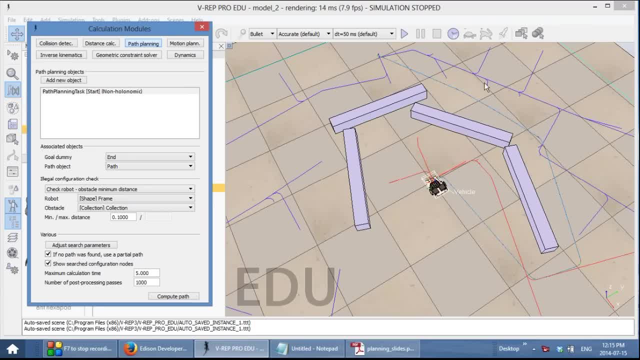 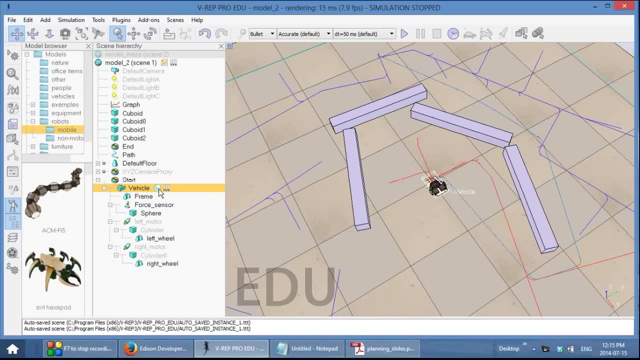 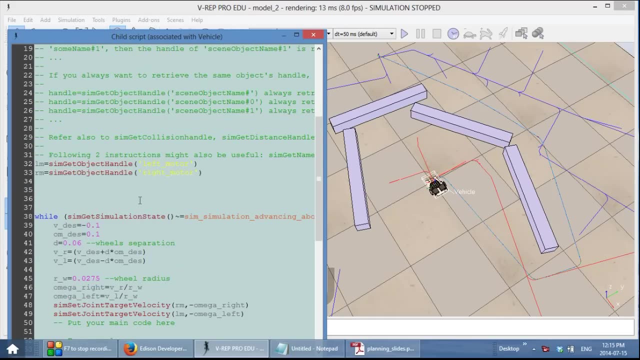 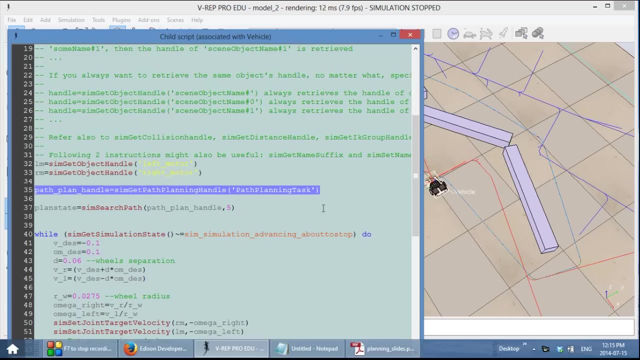 The System actually calculates Some sort of a path for you. Now. double click On the child script And you can add the following two lines Into your initialization, Just before the while loop. The first line Shown here Is: 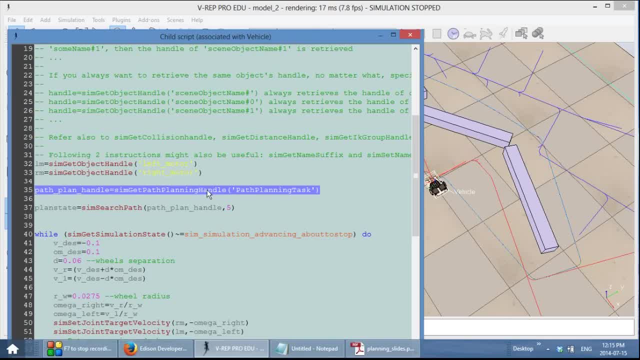 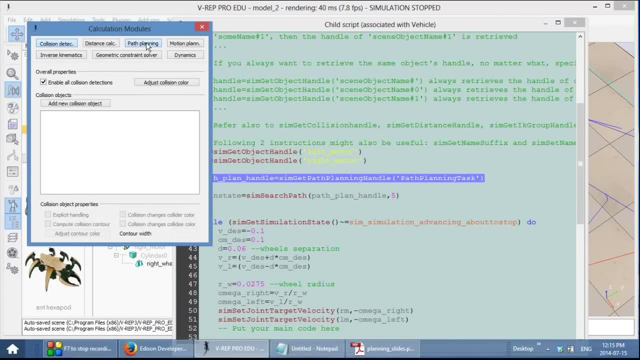 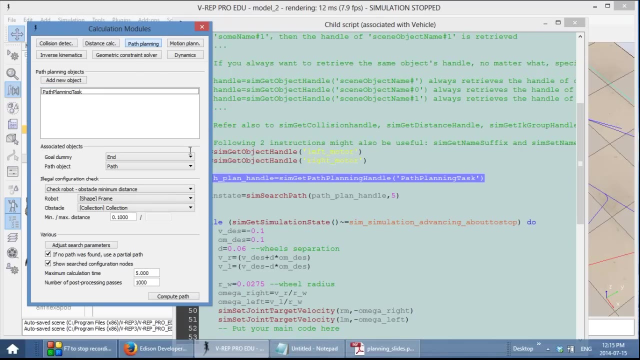 A function that gets a handle To the path planning object. Now here we have Path planning task, And the path planning task Is the following one right here, And if you double click on the name, You can actually change it To whatever you want. 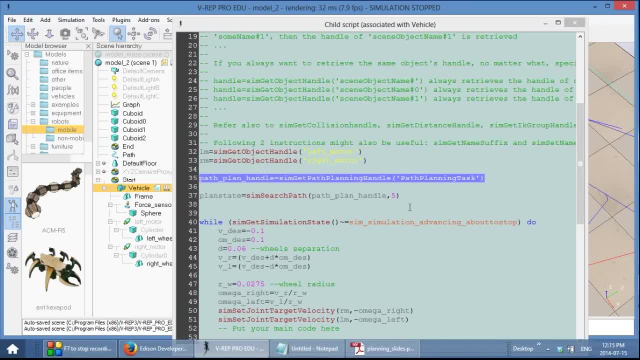 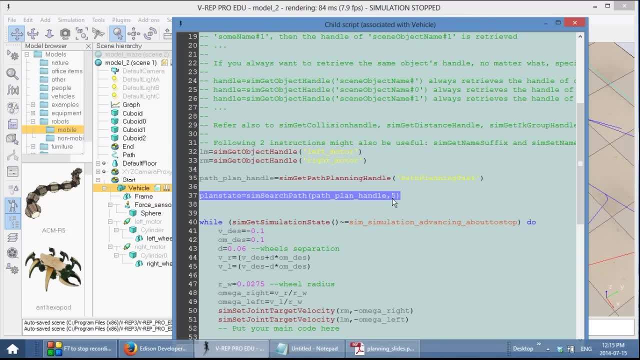 You can have multiple path planning tasks In the same simulation. Now the second line right here, Plan state, is equal to Sim search path, Path plan handle, comma five. This function, Sim search path, Takes in a path planning handle And then a maximum search time. 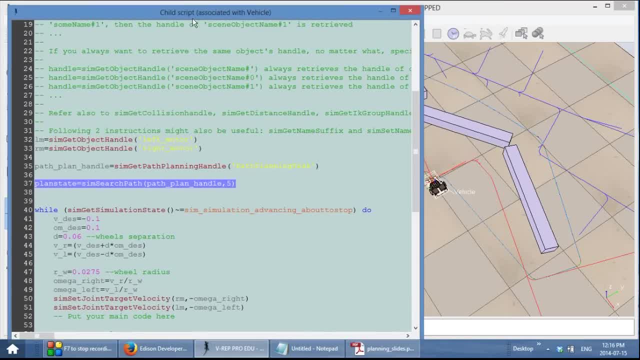 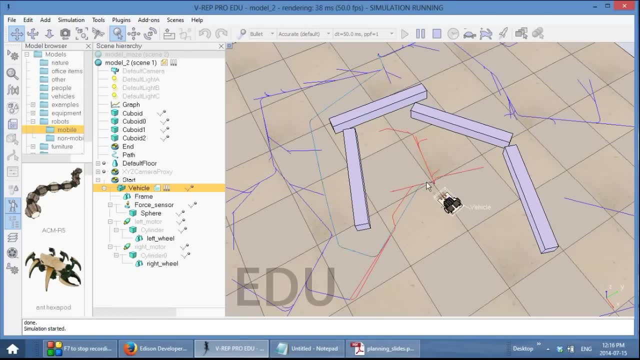 And then finds a- Essentially finds a- path. So what does that look like When we run the simulation? It recomputes a path At the beginning of the simulation. So what we want to do is: We want to have the system. 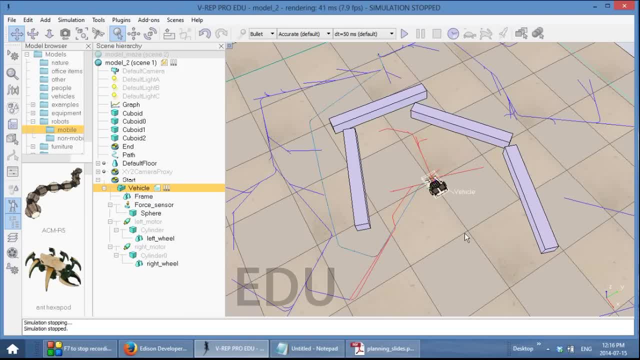 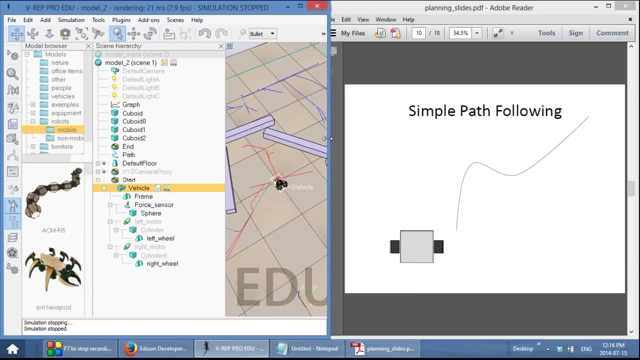 Calculate a new path Every time we restart the simulation. So now, how do we? What is our strategy here To control the robot? Essentially, this is what we currently have. We have a differential drive robot And a path. So now we have to decide. 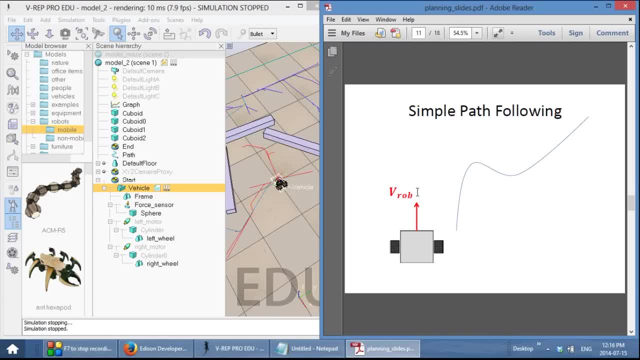 How do we follow the path? We would like the robot to go forward At a constant velocity, Which we call VROB. We can also, We have functions within VREP To find a point on a path. So what we do? 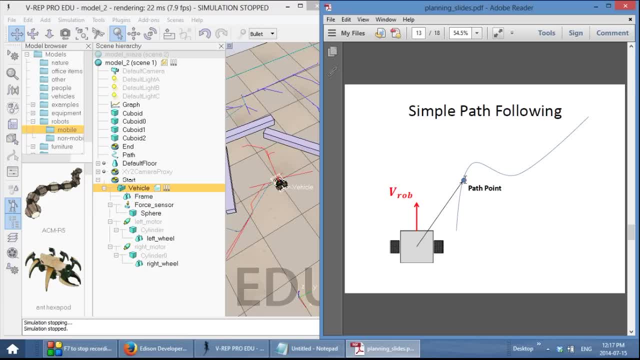 We draw a vector from our robot To our path point And this can tell us What exactly we have to do To navigate towards the path point. So what we do? We just use a simple proportional controller Where the rotational velocity of the robot 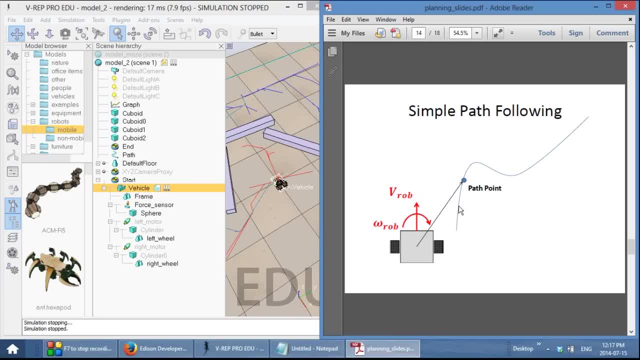 Is proportional to how far The point is to the side of the robot. So, essentially, When the robot is facing the path point, Our desired rotational velocity Will be zero, And the farther the robot is off to the side. If the robot was facing this orientation, 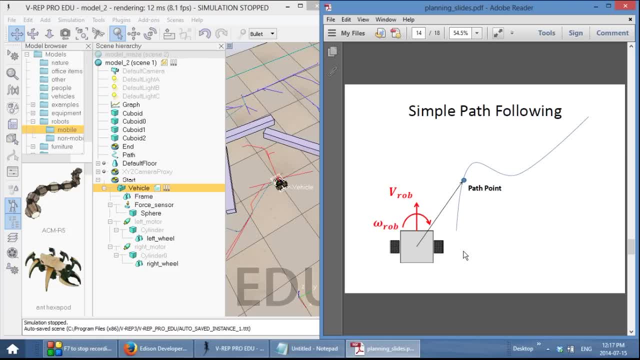 Then you would want A higher rotational velocity. So then, What the simulation Will do? It will drive the robot forward And increase its rotational velocity So that it points towards the path point. So then, what happens As the robot approaches the path point? 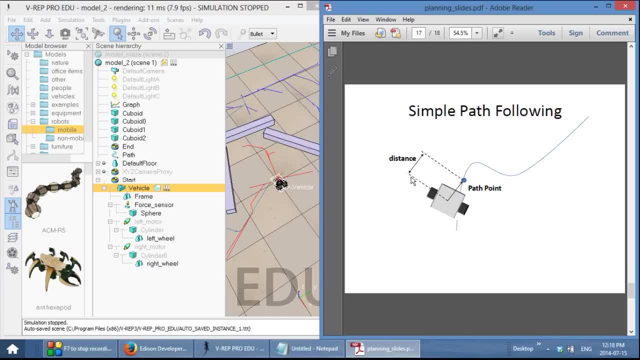 Once the robot Gets within a minimum distance, We can then go ahead And then select the next point Along the path, Like so, And then again We still have the forward velocity That we want to achieve To point the robot into the next point. 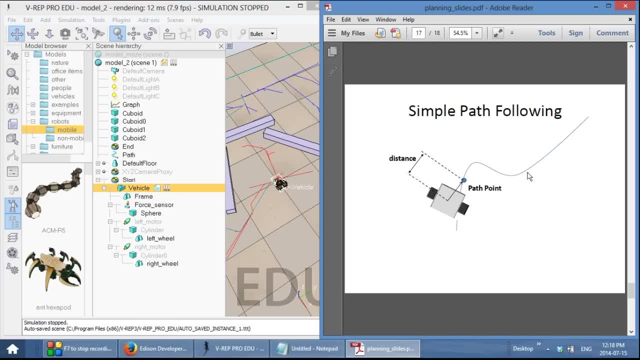 One thing you can see Is that this control strategy Is actually It works, but it's not great, Because you can see that this robot Will actually not go along this path. point One thing we can do Is we can actually reduce. 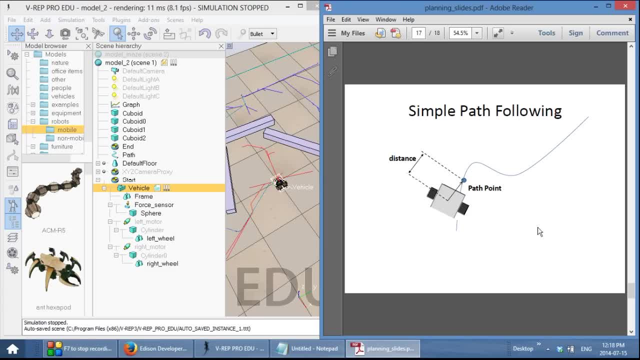 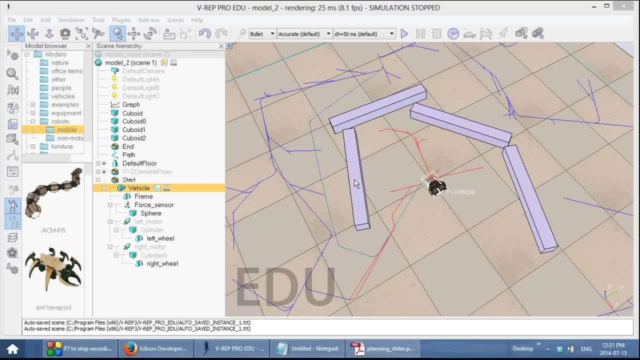 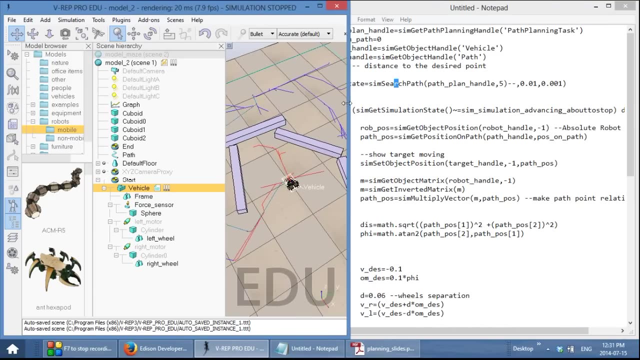 The distance between path points. So now Let's turn this strategy into code. In this Next little section, I'm going to write out the code line by line, And I'm going to explain What each of those lines does. I have here the pre-written code. 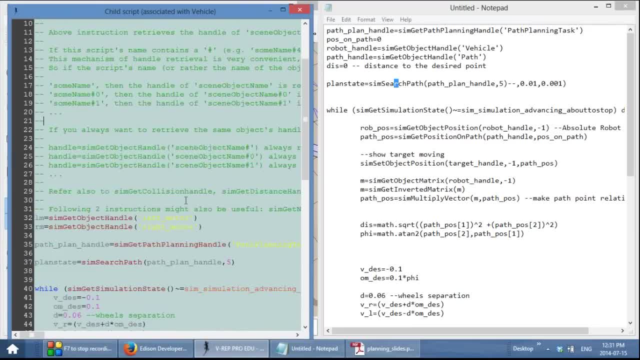 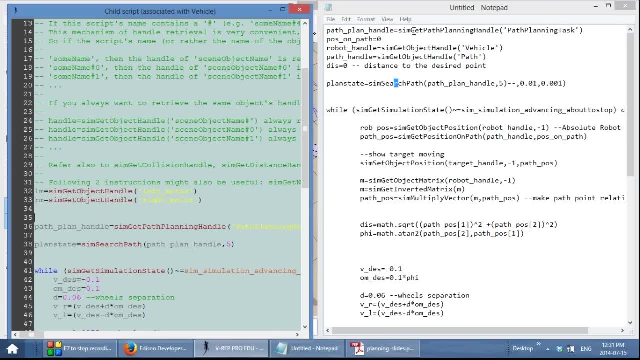 Which I will add into the script. We first begin With a couple of handles. We already have The path planning handle. Then we need something That's called a robot handle, Which is just a handle Towards The vehicle. Another thing we need: 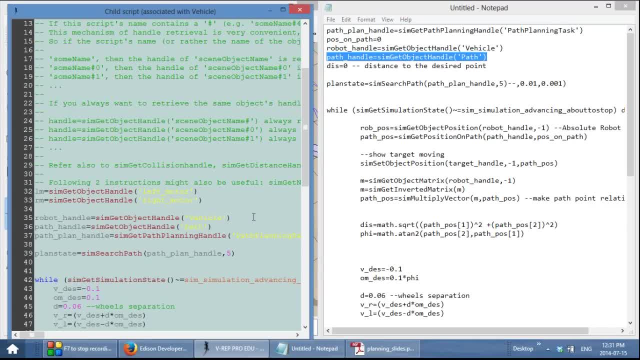 Is this path handle And this is a handle That points towards the path, And let's also define A few variables. The first one will be Position on path, Which I have abbreviated And we're going to set it to zero. 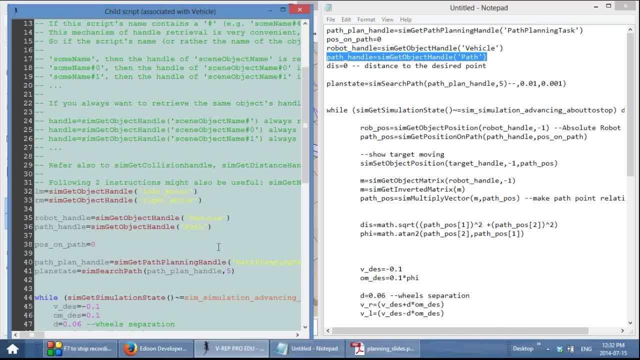 This will point us towards the Zero position on the path. The way VREP handles its path Is from zero to one, And we're going to Define a distance, Zero, Which is the distance From the robot To the. 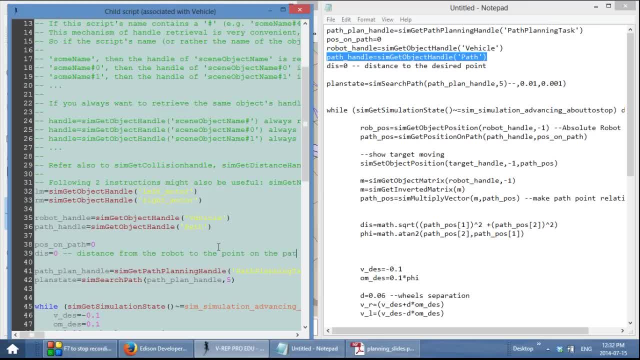 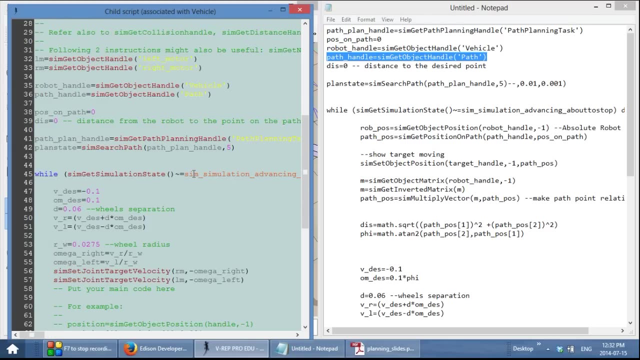 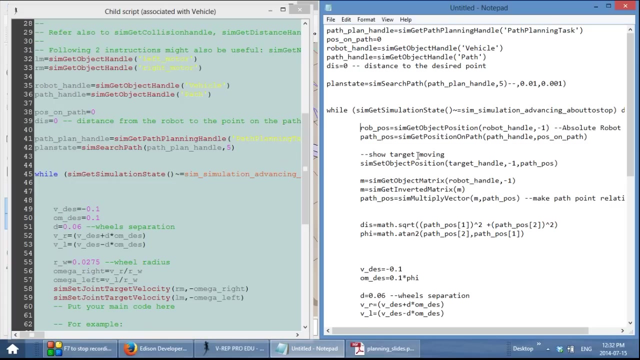 Point on the path. So This is enough of the Initialization. Now we can go into the while loop. The first thing we're going to do At the beginning of every loop: We're going to Retrieve the robot position, And we're going to do that. 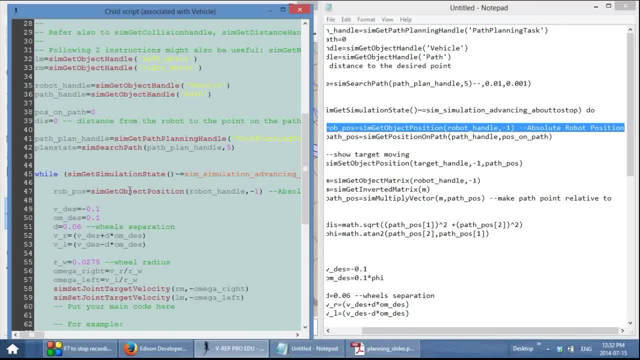 Using the command Sim, get object position Robot handle, Which is the handle that points Towards the desired object, And then minus one. Minus one retrieves the Position relative to the world Coordinate frame, The next thing we're going to do. 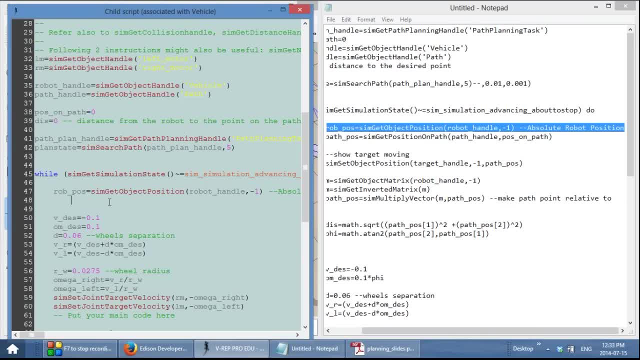 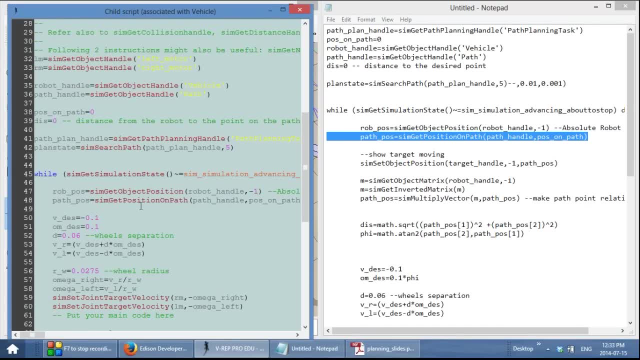 Is we're going to Retrieve a point on the path, Which we're going to Do Via the Sim. get position on path Function. This function takes in a path handle And a position on path That goes from zero to one. 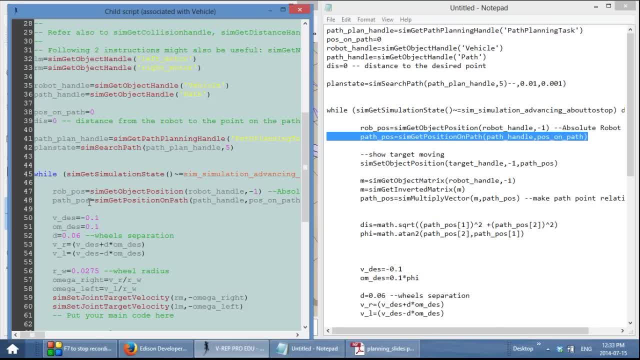 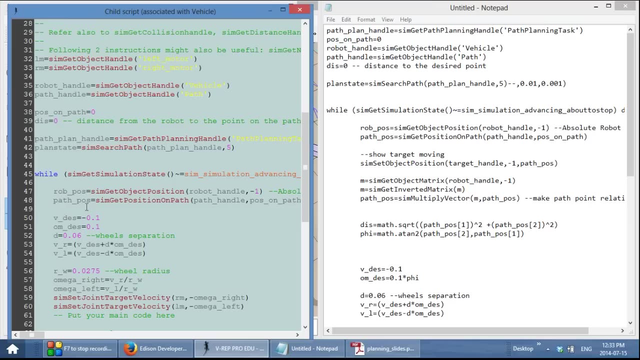 And it returns a path position Which is, I believe, A luau table. That has the position Actually, yeah, just the position In x, y and z. So another thing That we would like to add: We would like to advance the start node. 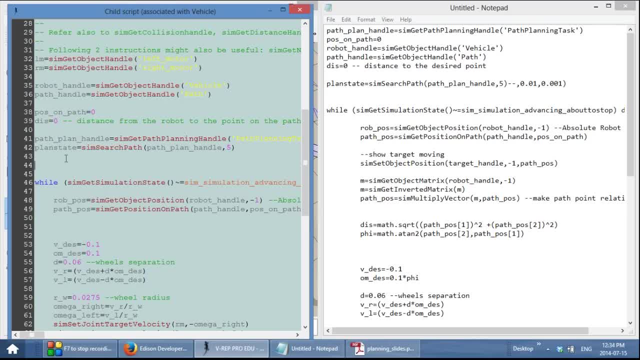 To show exactly Where the robot is pointing. So I'm going to Go ahead and add it now. I'm going to say: Start Dummy handle Is equal to sim, Get Object Handle And you can Select functions. 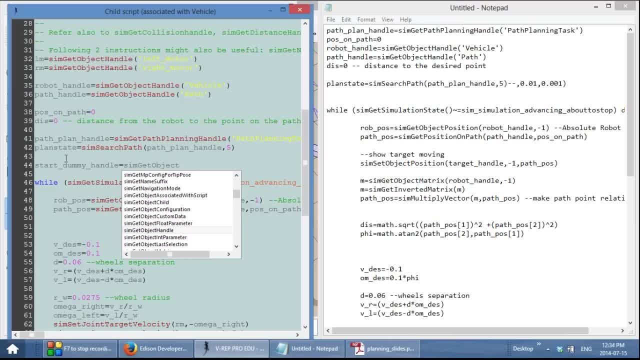 With the up and down key And then, if you want to use that particular function, You just press enter And the name of the dummy- The start dummy- was just start, And one thing we're going to do, We're going to place that. 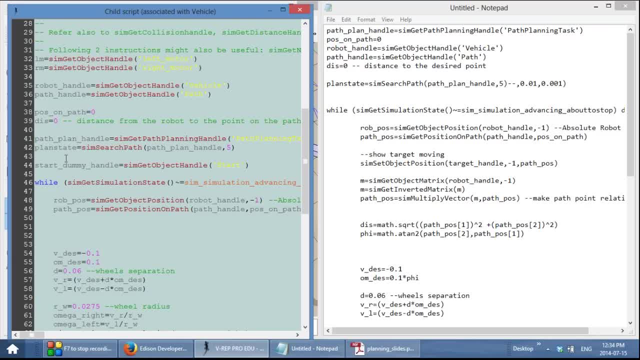 Start dummy To the desired, To the Position on the path, So that we can visualize exactly where the robot Wants to go. We're going to do that using sim Set Object position And then we'll say Start. 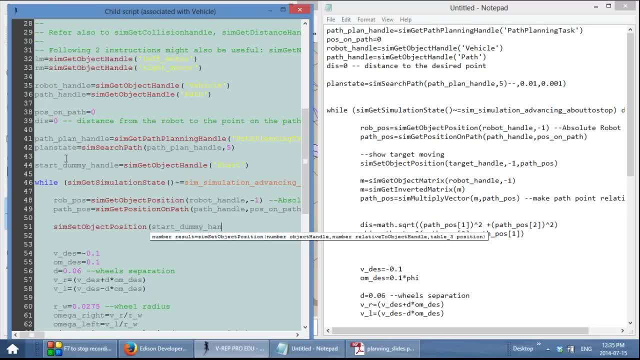 Dummy Handle And then minus one relative to the world, And This next one is The position, And we wanted to Place it on the path Position. So this will set the dummy At each iteration of the loop. It will set the position. 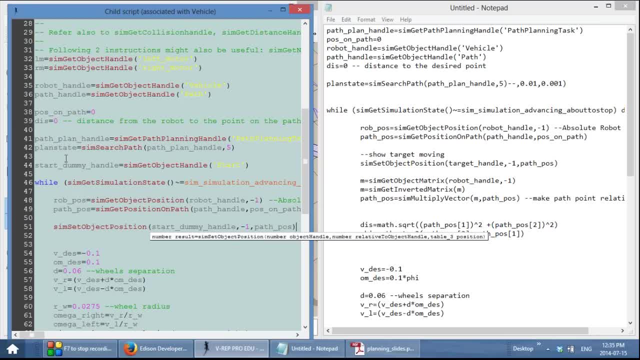 Of the start dummy Towards the position Of the point on the path. This next line, M is equal to sim Get Object matrix And then of the robot handle, Comma minus one. This Function Gets the transformation matrix. 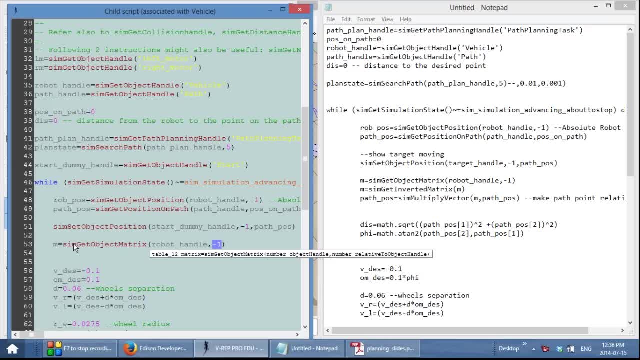 Of the point In the world coordinate frame, Because we set it to minus one And it transforms it To the robot position. We then want the inverse of this, Of this matrix, By using the sim Get inverted matrix command M. 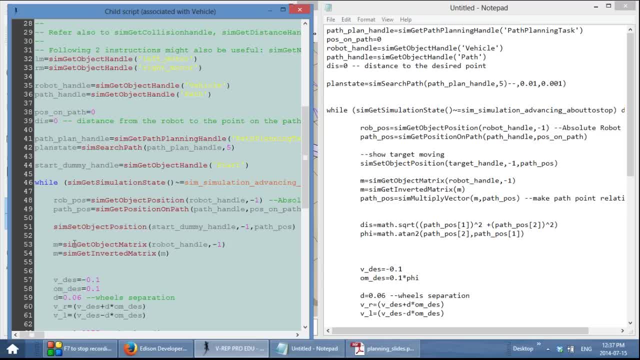 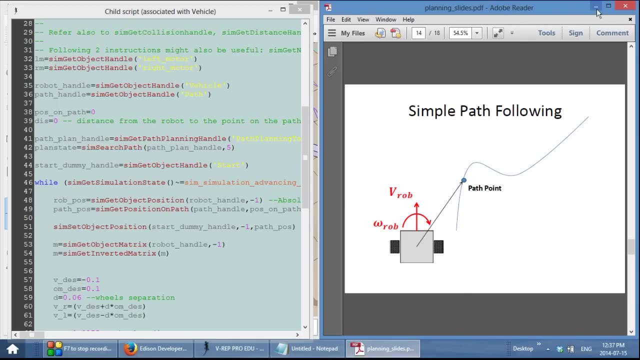 And now we have this matrix M In the environment. If you multiply it by M, Then you will get that position Relative to the robot. And relative to the robot is This vector right here? So what we do, We say: 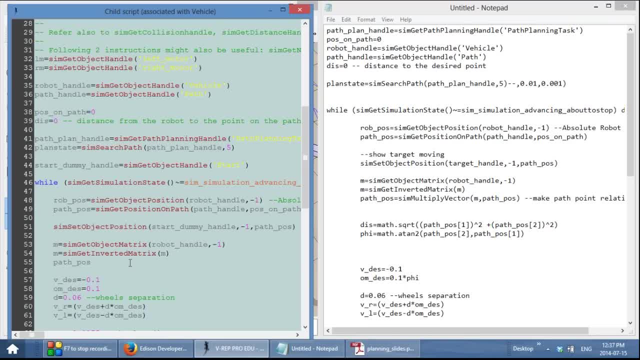 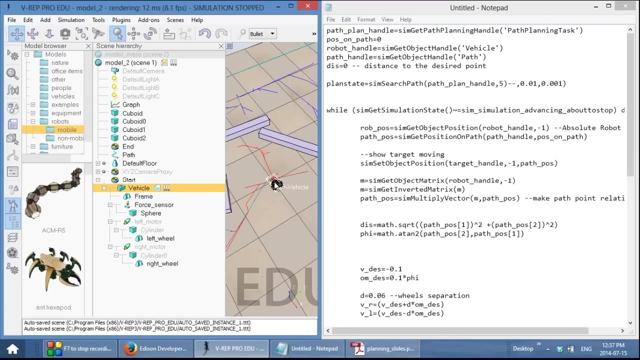 The path position, Which is the point on the path, Is equal to sim Multiply Vector And then M comma Path Position. So previously The path position point Was relative to the environment In 3D space. 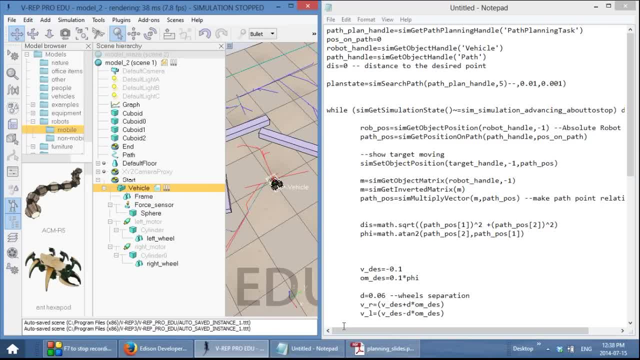 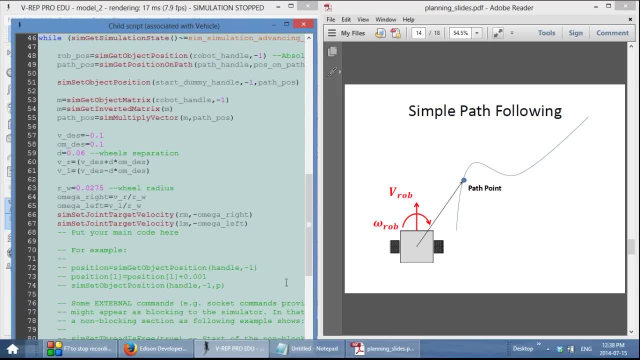 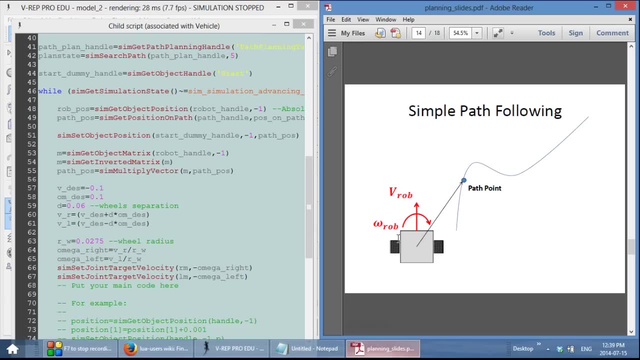 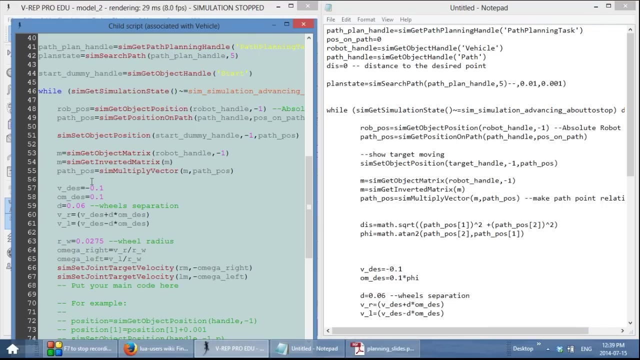 But after these three lines, It then changed it to be relative to the robot, So that it's like this: So This vector right here We can go ahead and Write our controller. One thing that we need to do: We need to first calculate the distance. 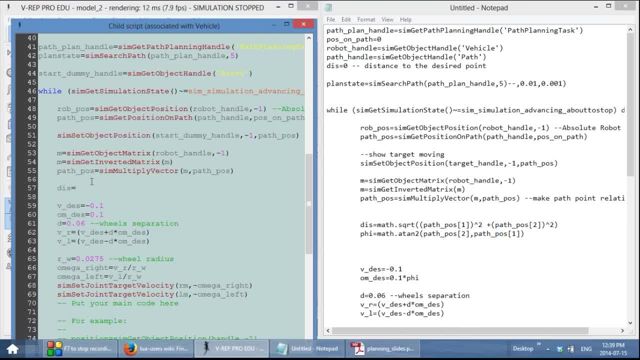 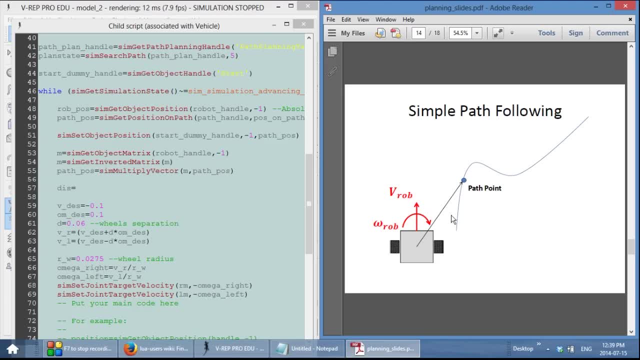 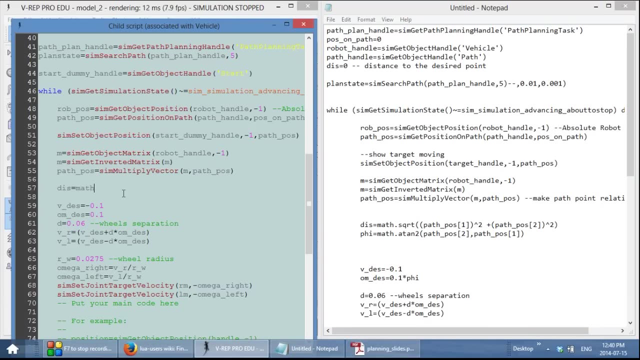 The distance between the robot And the The point. Now, since we're using a differential drive robot And the path point is on the ground, We will only consider the X and Y coordinates. So what we do? We use the math library. 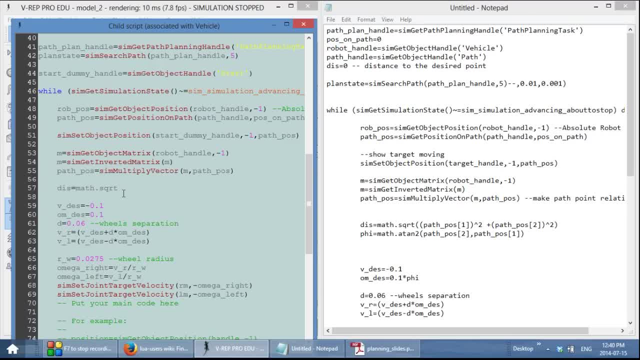 Math dot square root Of. And then we say Path position at 1.. So this will be the X Value of the vector Squared Plus Path position at 2. Which is the Y value Squared. So this should give us the distance. 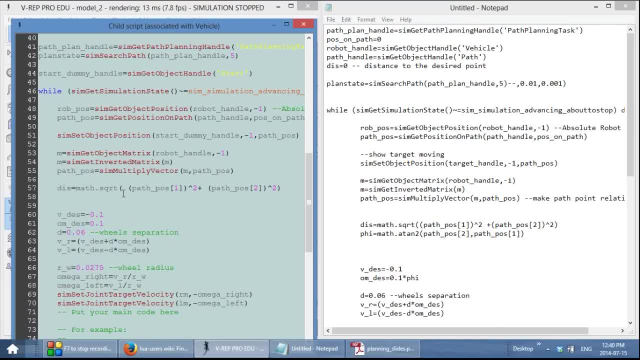 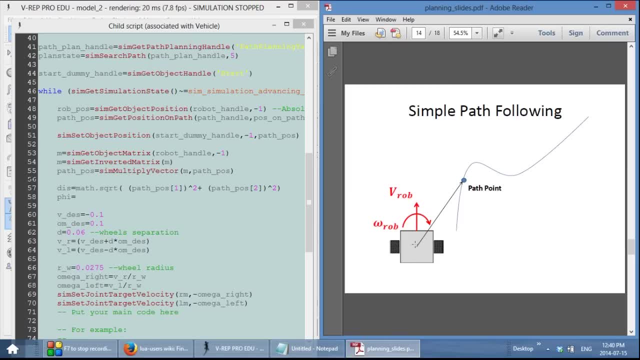 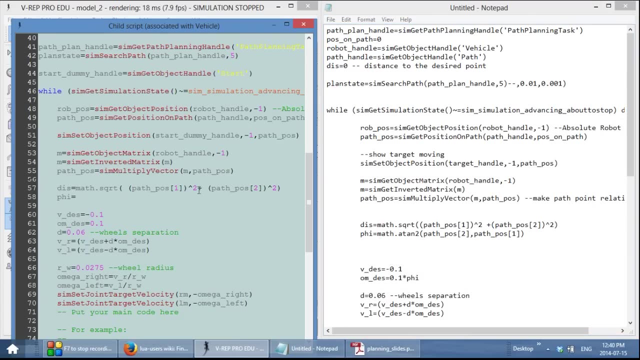 From the robot To our target point. And the next one, We're going to calculate the angle phi, And that's the angle That is made By the robot heading And the path point position. So again, We're going to use the math. 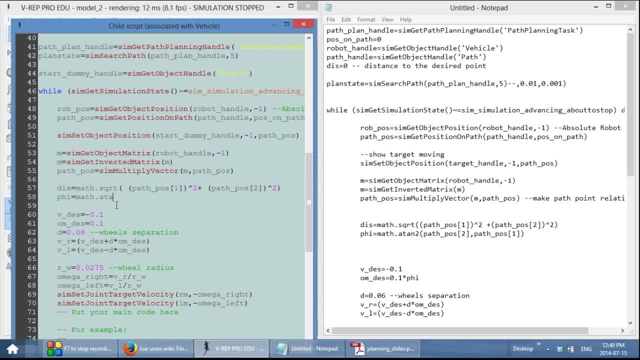 Library. So we go. math dot Atan2. Of. path position At 2 comma. Path Position at 1.. Alright, So as far as The desired velocity, We're just going to set It to a constant. 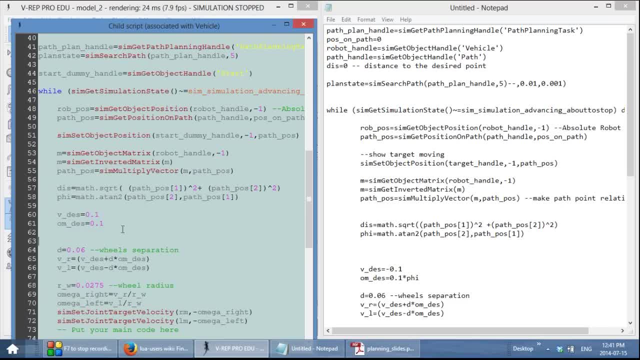 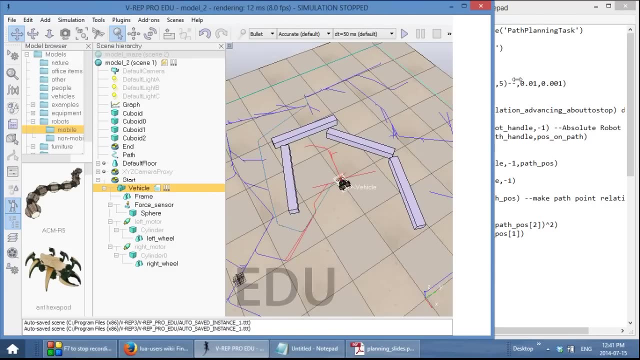 Of 0.1. Now the desired rotational velocity. We're going to set it proportional To this angle, phi. So let's say 0.1. Times phi And let's see What happens. So now, when we run the code, 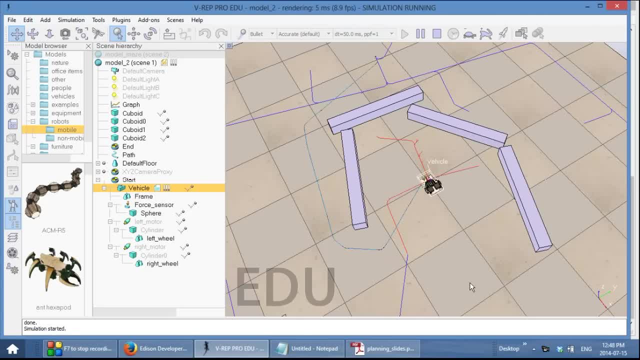 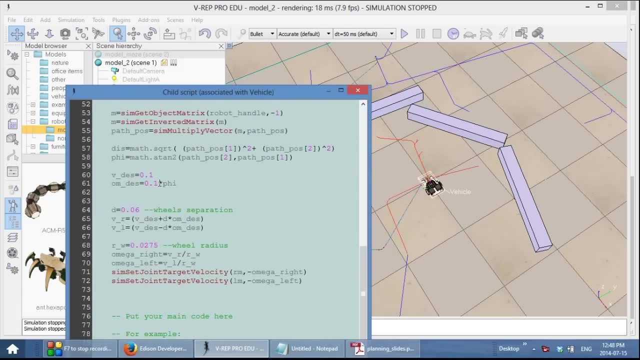 We'll find That the velocity happens, And that's attributed to multiple reasons. First of all, The proportional gain that we have Here Is a little bit too small, So let's set it to a little bit larger To make sure that the robot 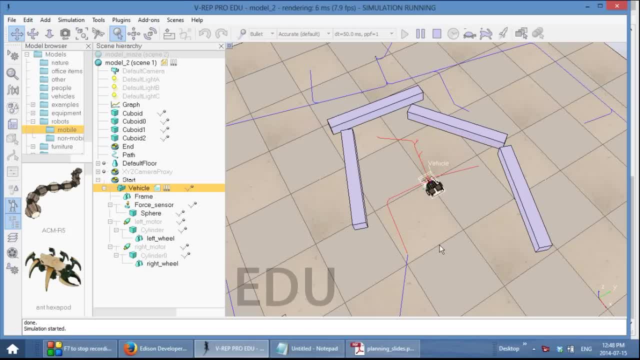 Turns more towards our desired point. And now you see that the robot Currently circles The starting point back and forth. That's because we have not Anything that advances Our path position to the next Location. In addition, you can see this thing moving along the path. 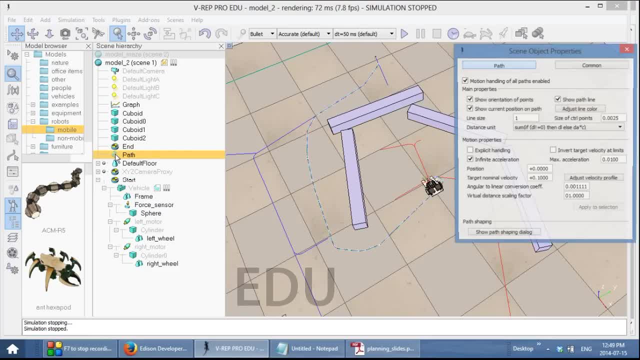 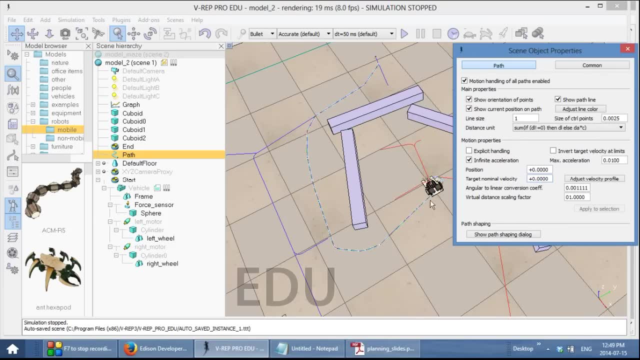 And that's just an artifact Of our previous work, Where we set The target nominal velocity to something. This does not actually affect Anything that we do right now, So I'm just going to set it to 0.. So now, when you run it, 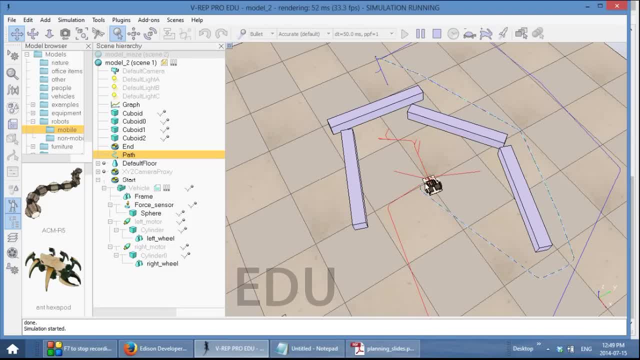 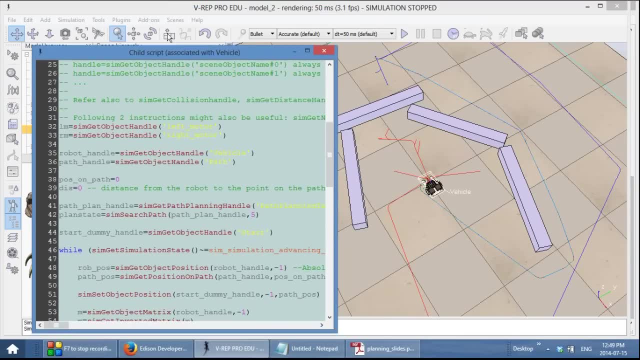 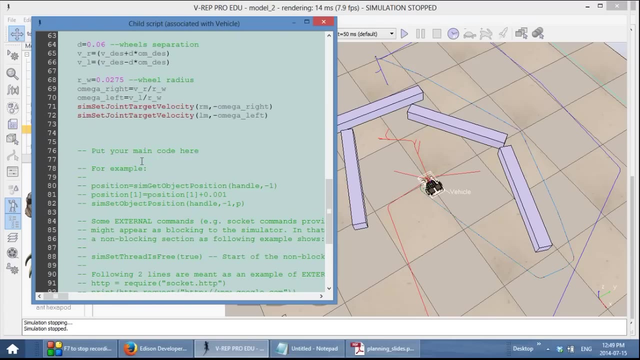 Again the same thing happens. The robot just kind of goes back and forth. So Let's add some code That advances our path position To the next level. So what we do here? At the very end of the loop We say: if 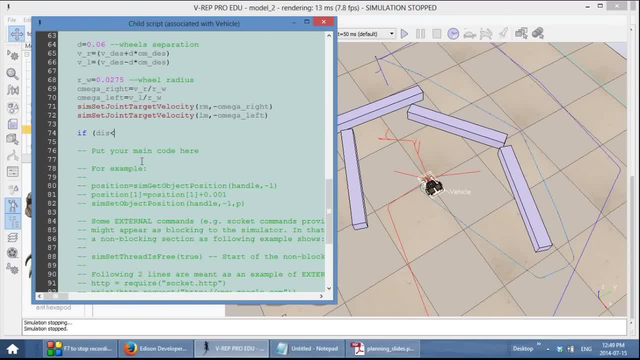 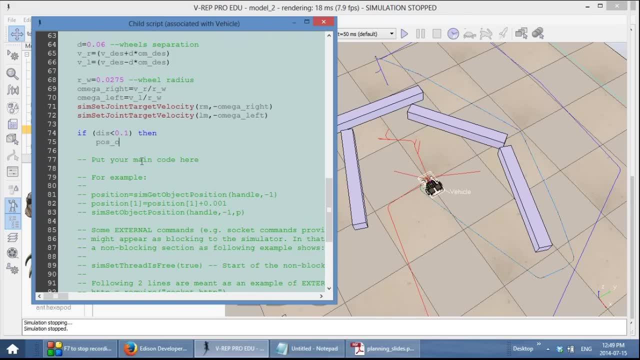 The distance is less than, And then this value you're going to have to tune, So let's say 0.1.. Then Position on path, And remember position on path Was a variable That goes from 0 to 1.. 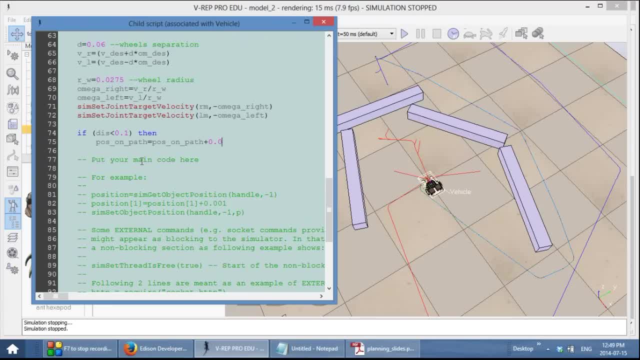 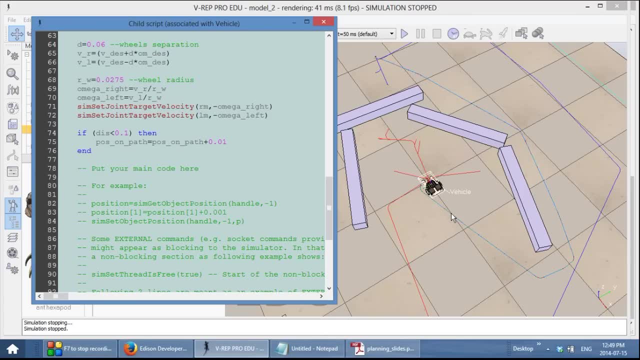 So we just advance it By, let's say, 0.01.. So now, If the robot gets within 0.1 meters of a point, Then it goes on to the next one. In addition, One thing that we should do: 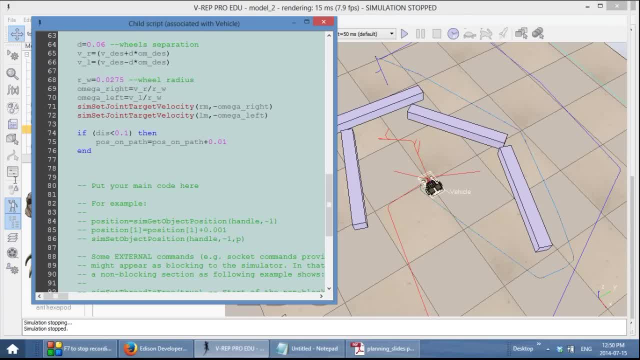 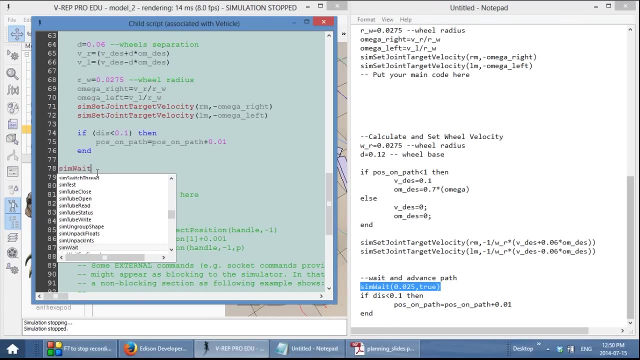 Which is Good practice when you're doing Any kind of simulation. We want this simulation to happen At a fixed time step, So we're going to add in The following command: Sim weight And then The time in seconds. 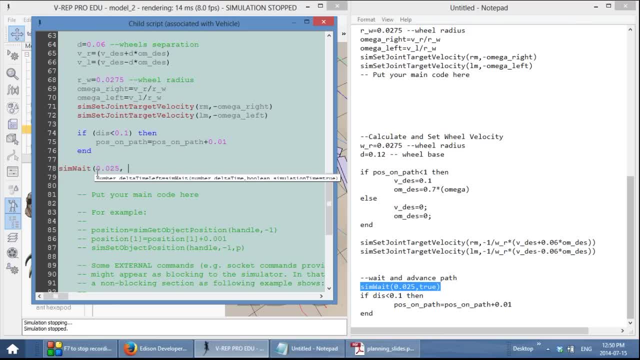 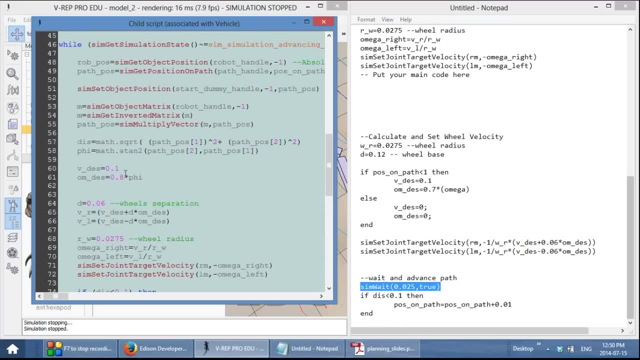 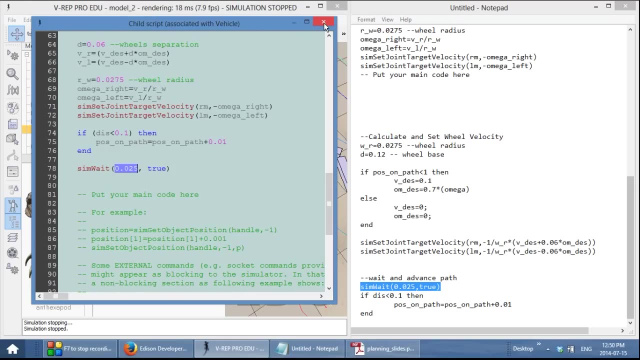 So let's set it to 0.025.. And then say: Simulation time: true, So essentially now This control thread Is going to run at 50 hertz, And this is just A good practice, because you always want Your control systems. 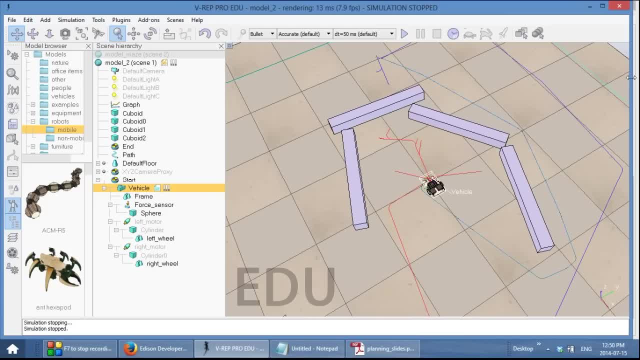 To run at a fixed rate. That's a desirable Thing to have, So let's run this code now And now. You can see The target Note advancing along And you can see the robot Roughly follow the path. 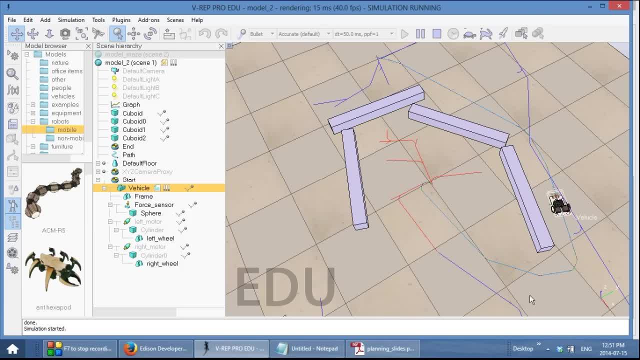 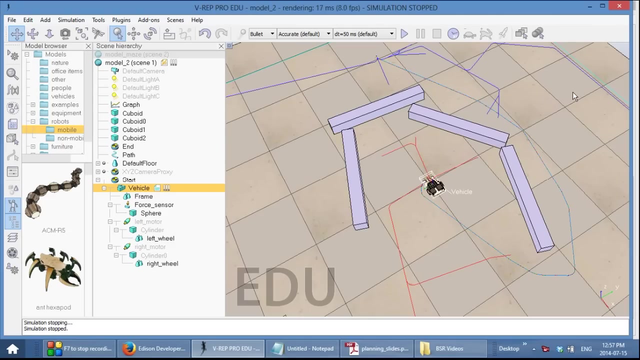 That we have laid out. Now One thing you will notice: As the robot gets towards its end, You'll see that It actually just Starts going. We need to add a stopping condition For the robot to know When it has reached. 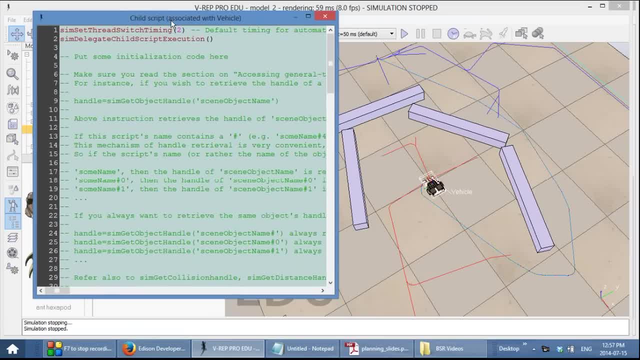 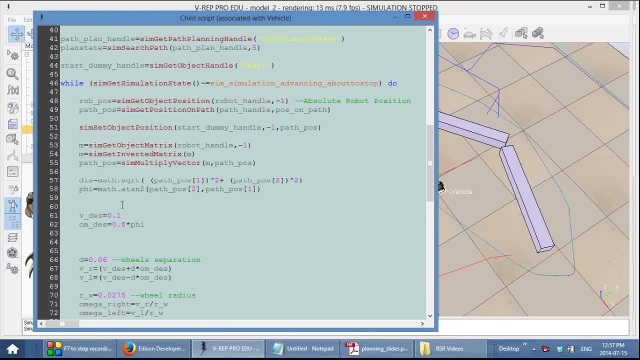 Its final position. We can do that In the while loop Via the position on path variable. We will set a condition Right here Where it sets the desired velocity And rotational rate. We will say: On path Is less than one. 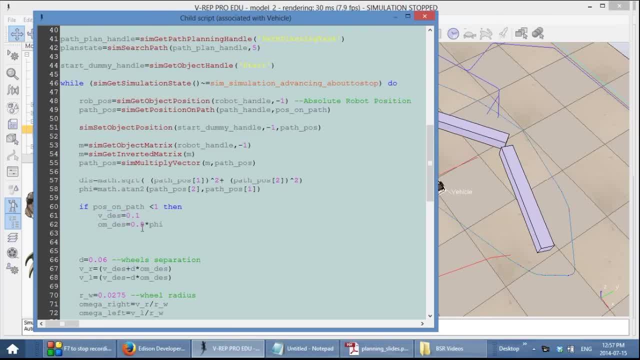 Then set our desired velocity To zero, point one, And our desired rotational rate Proportional to the angle. Otherwise, if the position on path Is equal to or greater than one, Set velocity desired Equal to zero And our rotational rate. 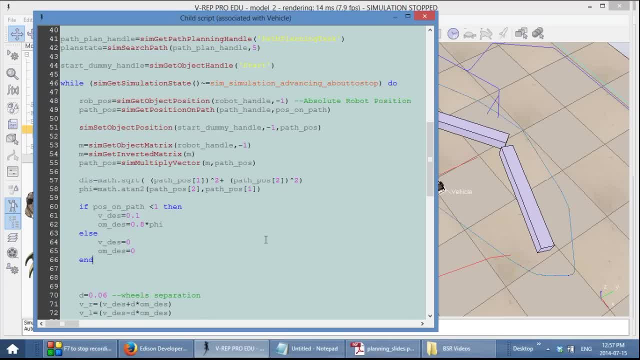 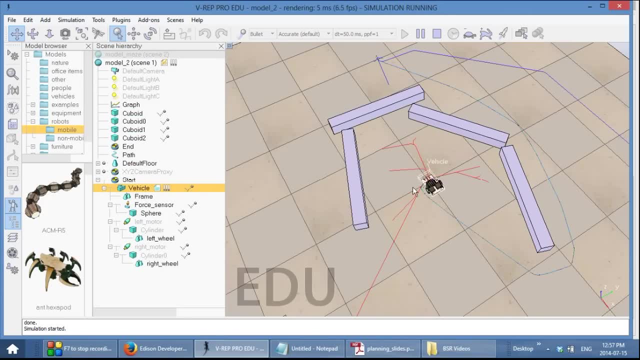 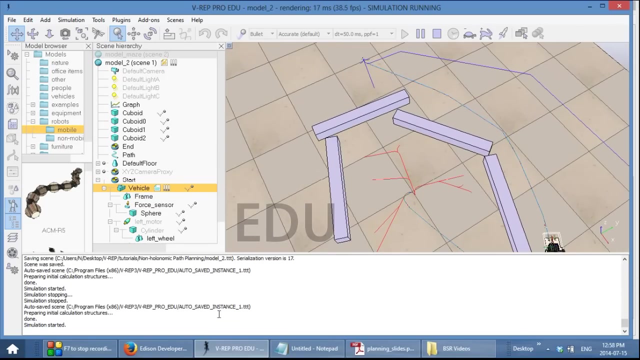 Also equal to zero. So now It should go ahead And Move towards the point And then eventually Reach its final position. One thing I should note While we wait for the robot To reach its final position Is that if at any point 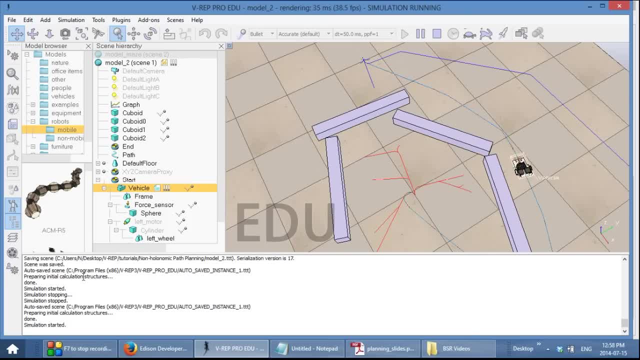 The simulation does not behave How you want it. Check down here To make sure that you don't have any errors Or typos That VREP will tell you about, And then you will see That the robot just kind of moves along. 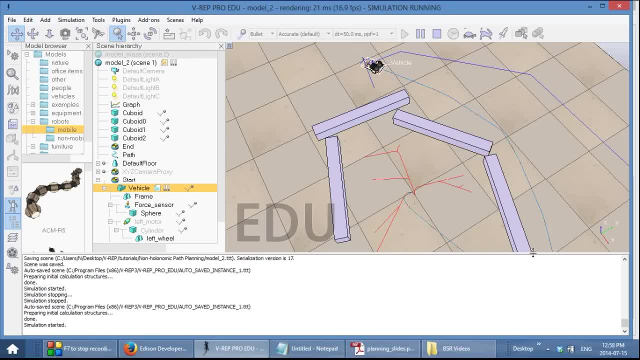 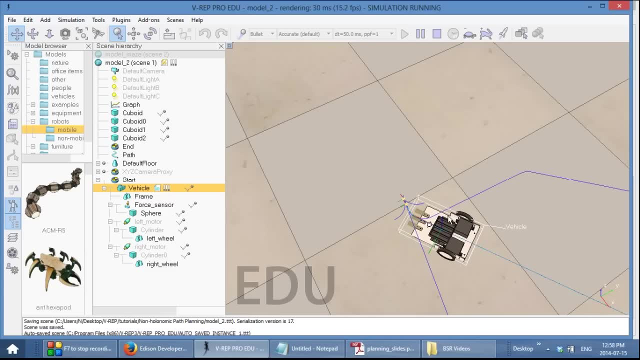 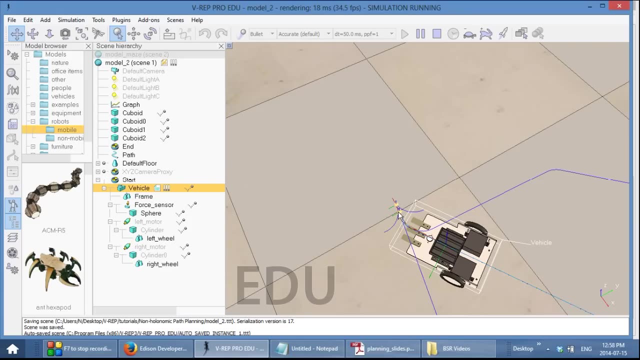 And then, once the position Is greater than one, You will see that the robot stops. Now this controller Is not really All that great. It sort of works, But you will see That our robot did not actually Meet its final configuration. 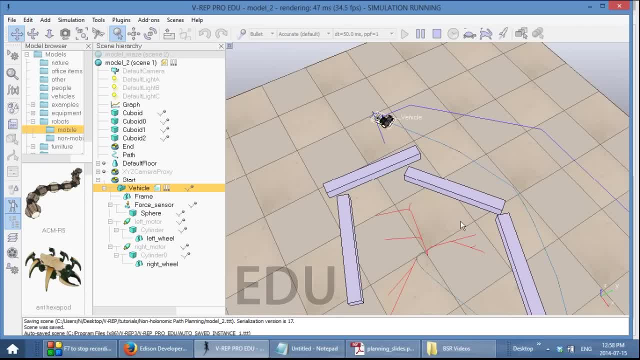 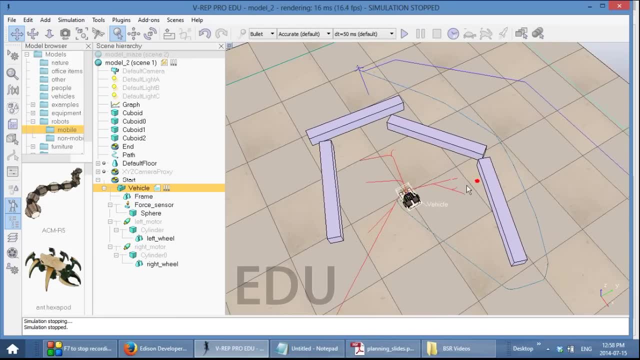 But that's because This is just kind of a Controller that was put together By a more advanced controller. I would suggest that you look into path planning Or more like Trajectory, following algorithms That are a little bit more advanced. 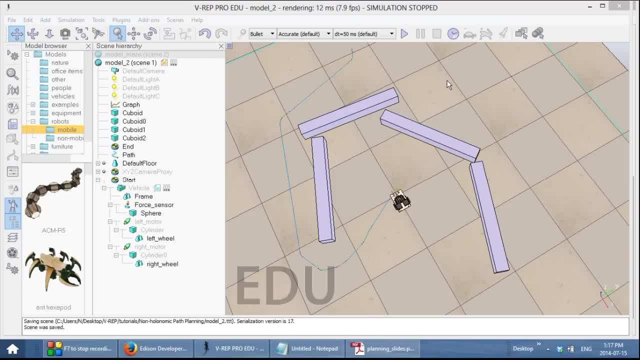 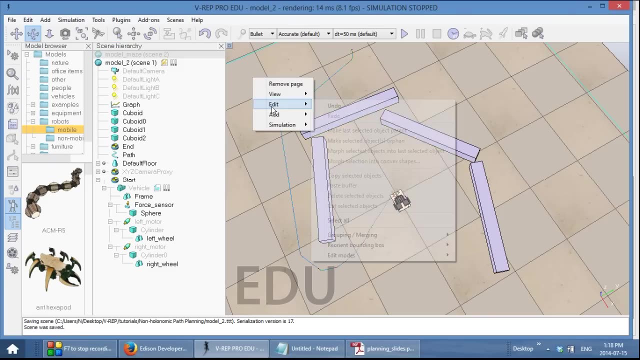 As a final addition to the simulation, We want to add A method To evaluate how well the robot actually Follows the path That has been calculated for it. We are going to do that In the environment: Right click anywhere in the environment. 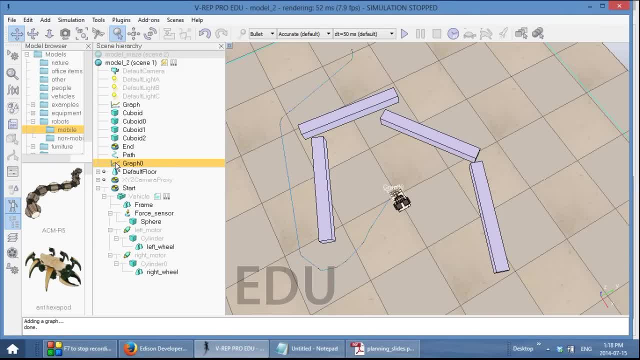 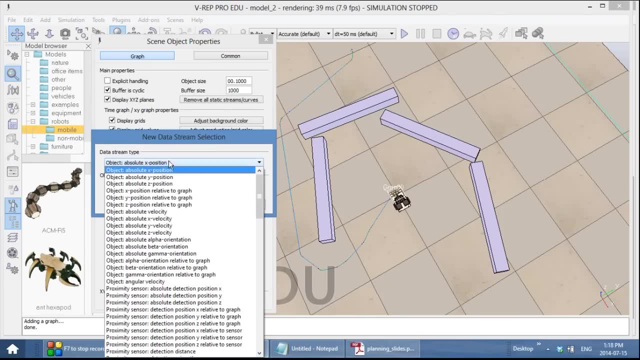 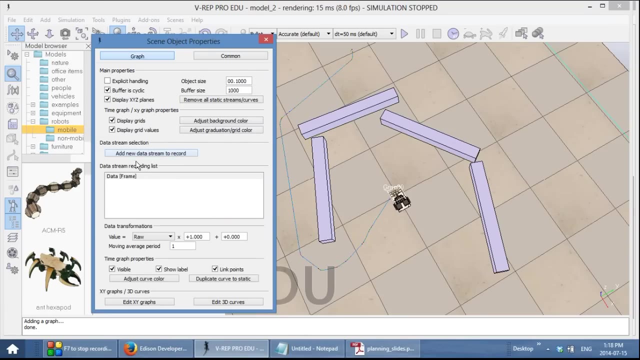 Select add and then graph. Double click on the graph And then select Add new data stream to record. Select X position Relative to graph And then select frame And then make sure To rename this into X, Because we are going to be using it later. 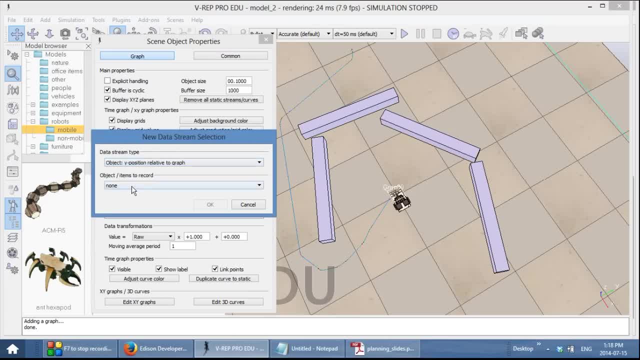 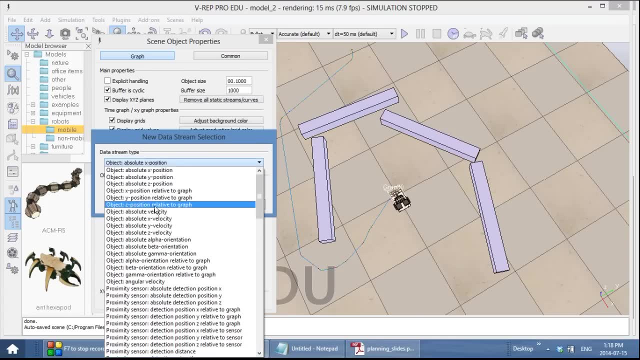 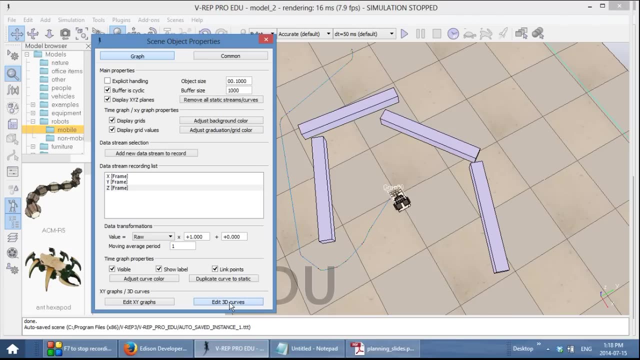 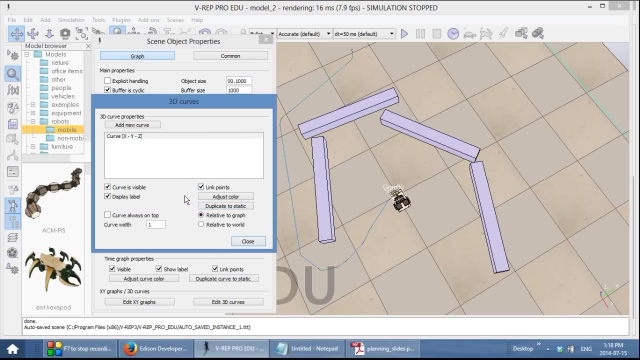 And we have to identify it by the name. Do the same thing for the Y And the Z position. So then select, edit 3D curves, Add new curve, And then here for X, Y and Z, Select the appropriate counterpart And make the curve width. 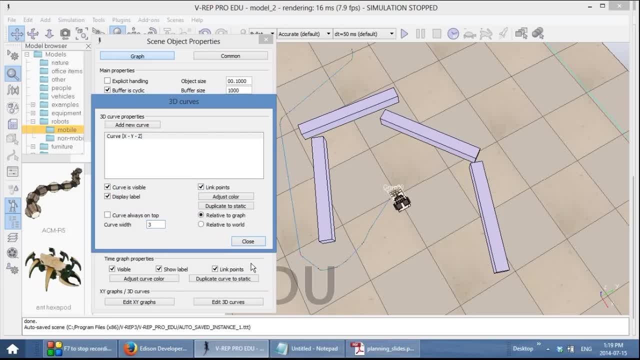 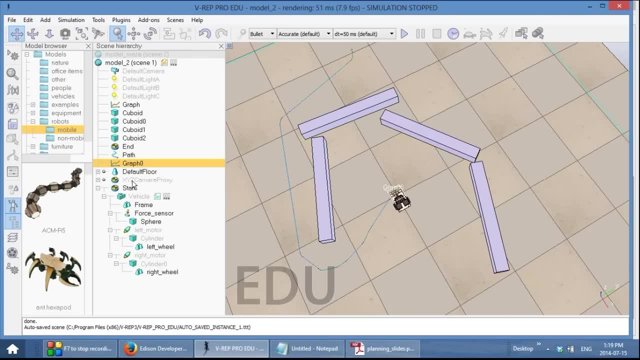 A little bit wider. For example, select it as 3.. You can also adjust the color, But that is not important right now. Then one thing we have to add: We have to actually make sure that The graph and the frame Are in the same location. 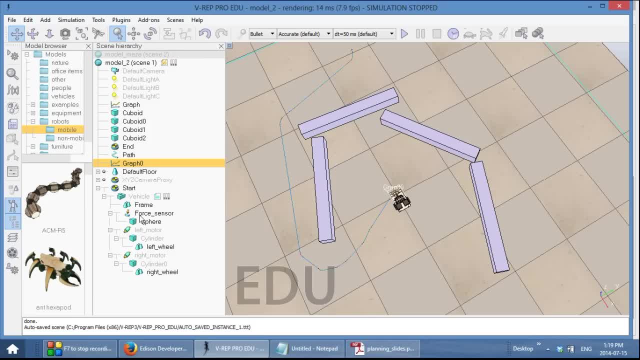 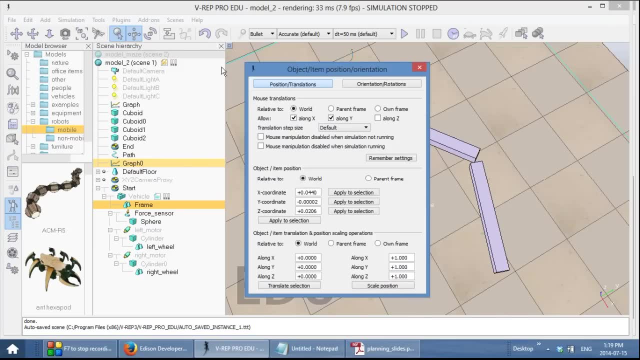 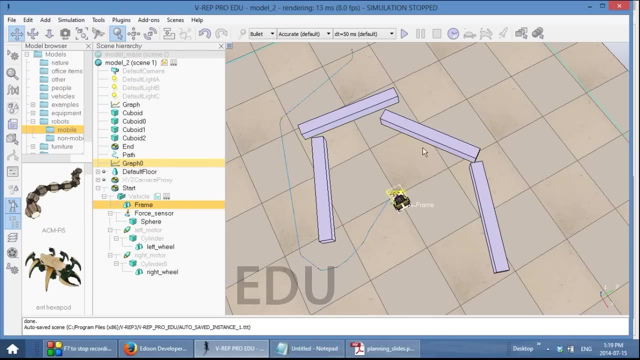 So select, click on graph And then with control- Well, with control held- Click on frame, Then select position And click apply to selection For the X, Y and Z. So now, when you run the simulation, You will find that the robot. 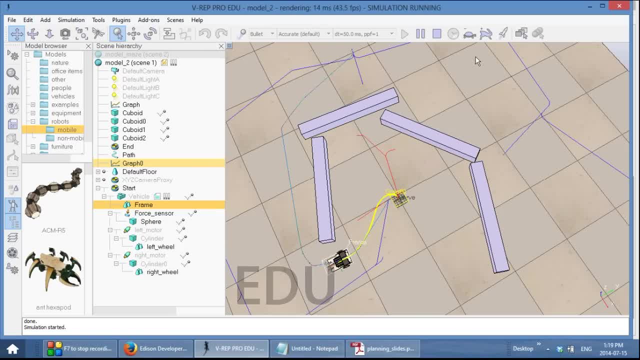 Should just move along And you will see the path drawn out behind it. We are going to do just a few Improvements. You can see How well it actually Follows the path, But we want to be able to Well. 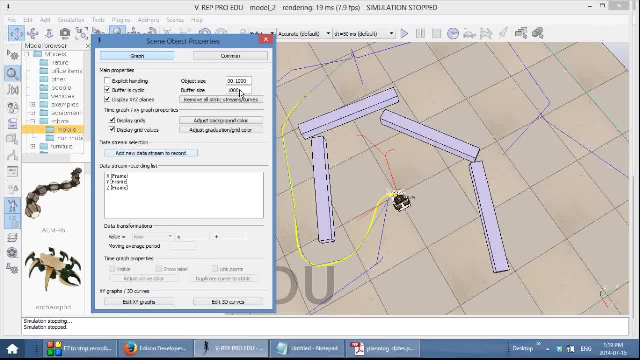 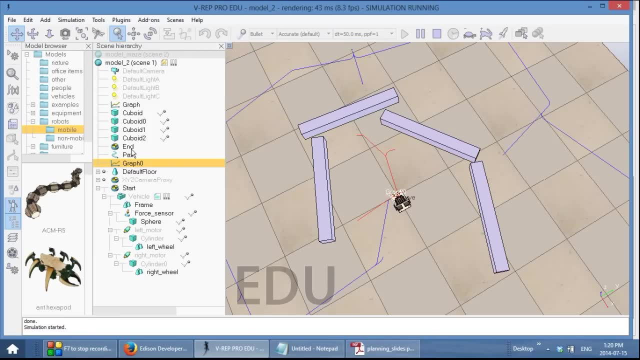 Let's clean it up a little bit. Double click on the graph And then select display X, Y, Z plane. This will hide the graph From our simulation, So we don't have to see it. In addition, We don't really. 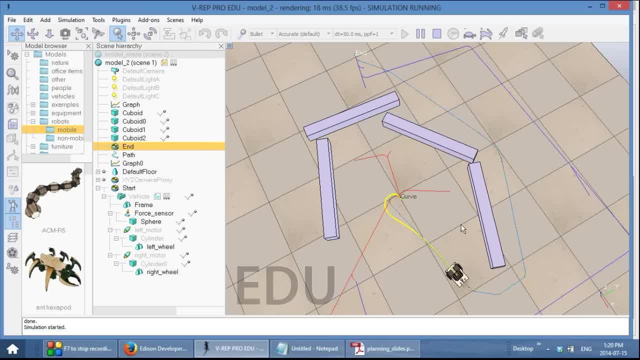 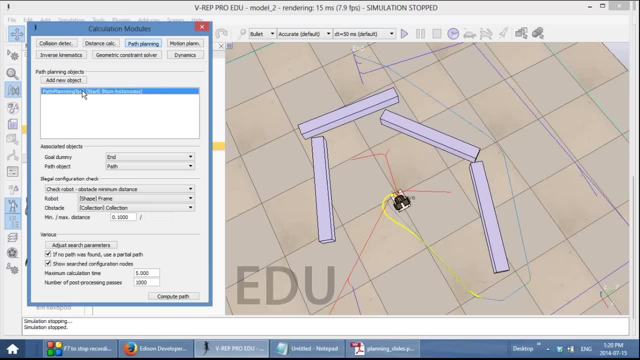 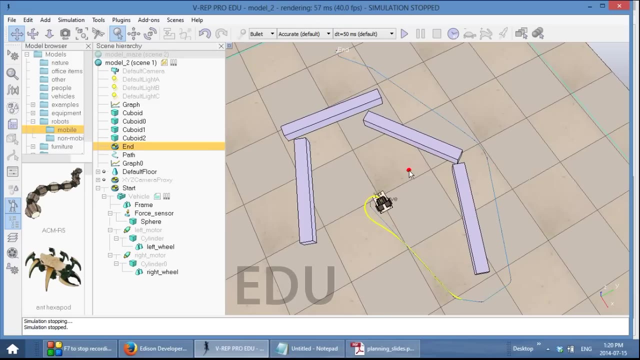 Need to see all of these Paths that were considered But were not actually used. So click on The calculation module properties Under path planning And then deselect. Show search configuration nodes. In addition, We want to have a true top view. 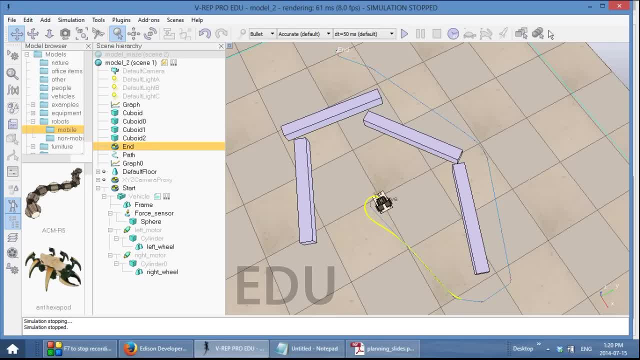 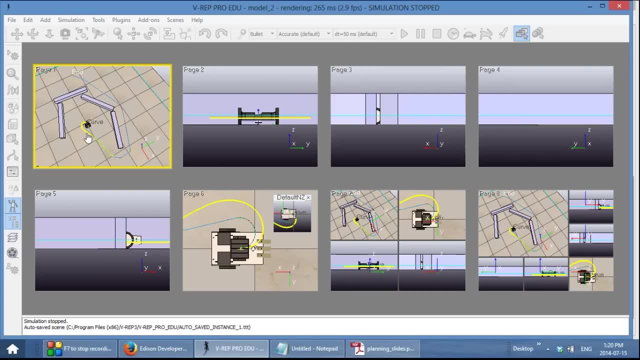 Of the robot. So this allows me to introduce A page selector, And here you can see Your default view That we have been working with. But here there is a couple of views, For example. this one Is the Y Z view. 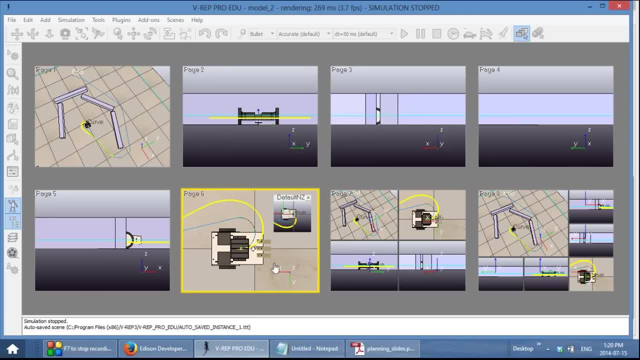 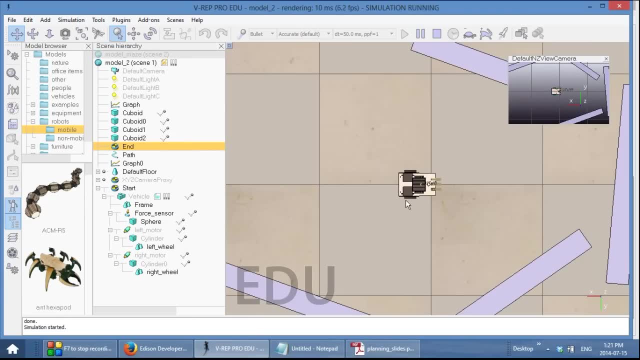 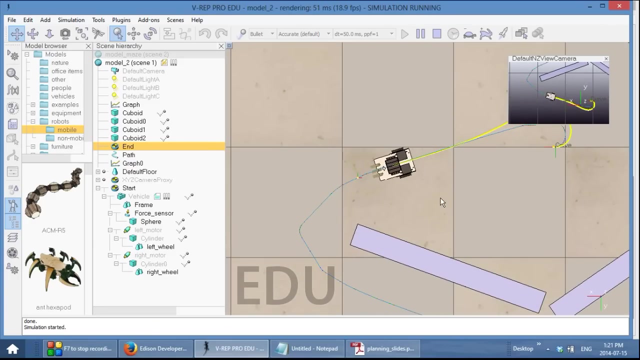 X- Y. So we are looking For this view right here, Which is looking straight down On the X Y plane. So now, when you run this simulation, You can see exactly How well the robot Actually follows The path And, if you want, you can play around.